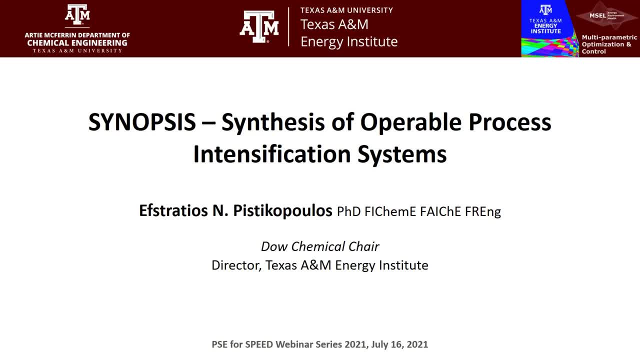 This is a project in the area of And under the auspices of the ASCHE, and there is a manufacturing USA institute. there's a manufacturing USA institute called the Rapid Institute on Process Intensification. This is a project in the area of. 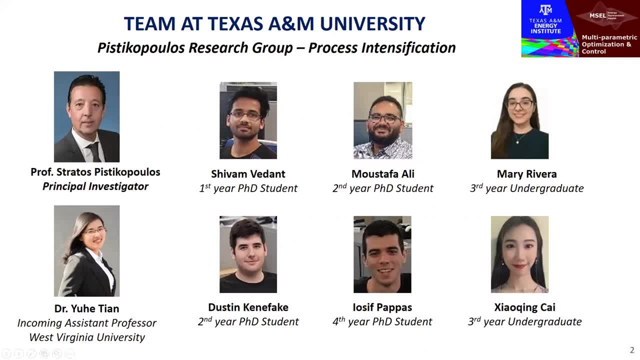 And under the auspices of the ASCHE, and there is a manufacturing USA institute. there's a manufacturing USA institute called the Rapid Institute on Process Intensification. So I would like first to acknowledge the process intensification team. It's an intensified team. 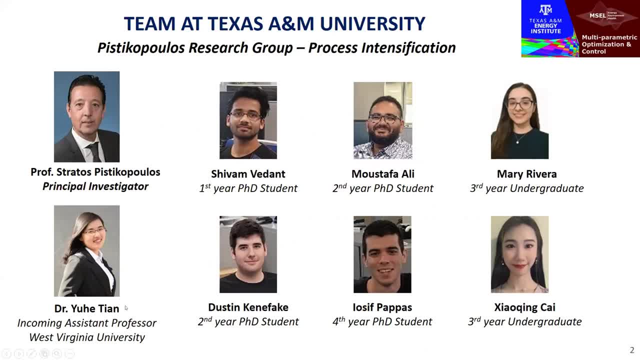 So I would like, in particular, to acknowledge Dr Eugen Tian, or I should say professor now. Eugen Tian, who is, in less than two weeks' time, going to be an assistant professor, started as an assistant professor at West Virginia University. 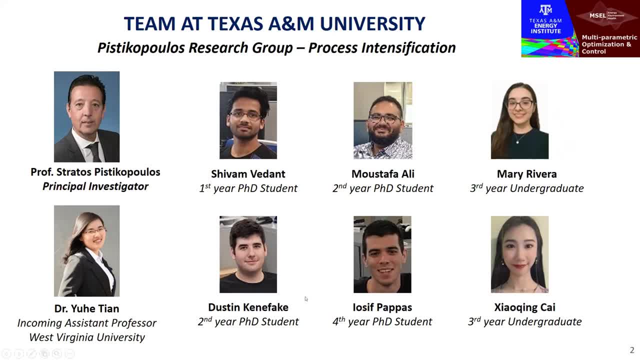 And you can see the members of the team. in particular, you know the SIVAM Bedan, who has worked together with Mary on the software side, on the synthesis front, and the, you know Dustin and Lucy, for the operability. 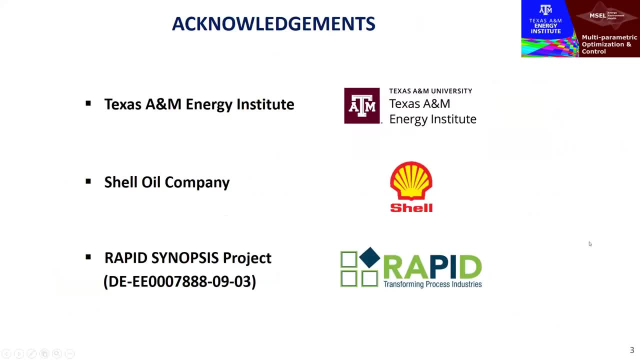 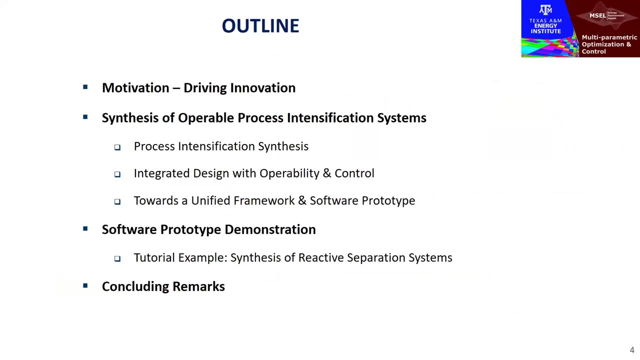 Mustafa and Ziad King on the safety aspect. So I would like also to acknowledge, apart from Rapid's cell, which has been instrumental in finding major components of the developments I'm going to describe. So a little bit I'll talk about, although you know, you have been already familiarize yourself about, you know driving innovation and how process intensification can become a driver in this space. 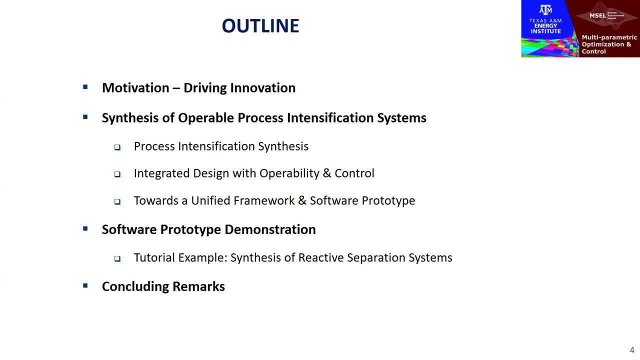 I'll describe a little bit about the synthesis framework in a way to follow, And I'll also show you fresh from the press for the first time: open our software. you know, like a four or five-minute hour software prototype demonstration. 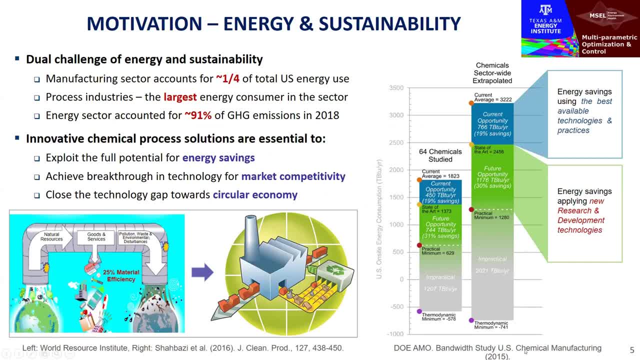 So time, obviously, we have been talking about the some of the challenges that modern society is facing and clearly energy and sustainability is at the forefront, and the key question is how we can drive innovation for energy savings to, you know, like encompassing aspects of circular economy. 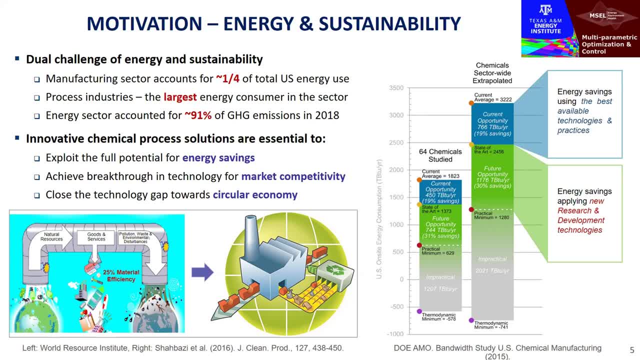 novel renewable energy technologies and the like you can. perhaps you have seen already the highlights in European Union. you know they are aiming towards by 2050 to face out, you know, the conventional fuels in the form that we have been talking about. while this is like an ambitious plan, 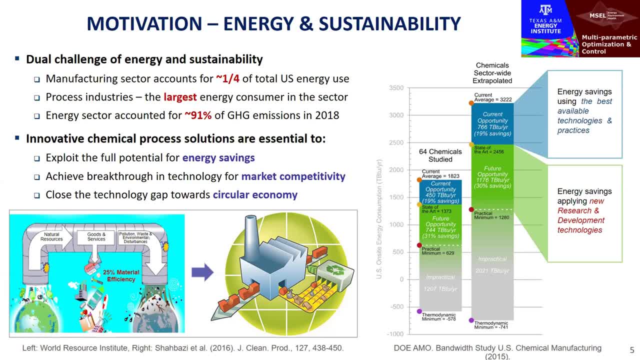 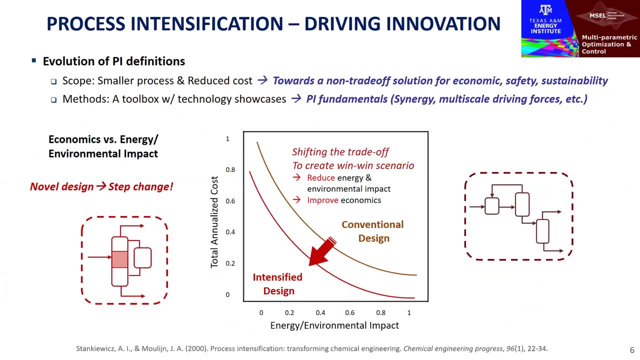 you know, the question for us in the process systems community and generally the scientific community is how we can drive innovation for energy savings. to you know, the key question is how we can. what are the key players towards making sure that these targets can be achieved? And processification is one of these key components that can drive innovation in many ways. 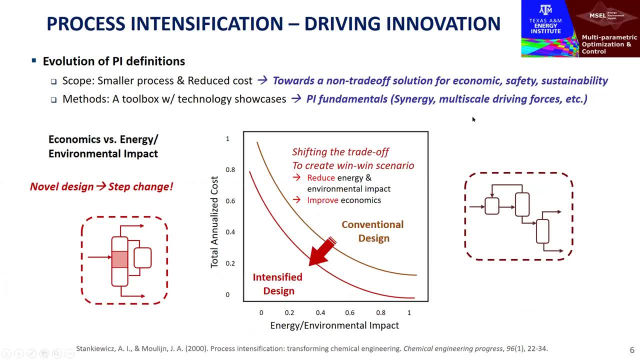 because it can achieve win-win scenarios in terms of both cost and energy and environmental impact by changing the conventional design, the structure, the design characteristics, towards innovative type of step changes. right, And you know obviously you have seen already exams in the context of the webinars. 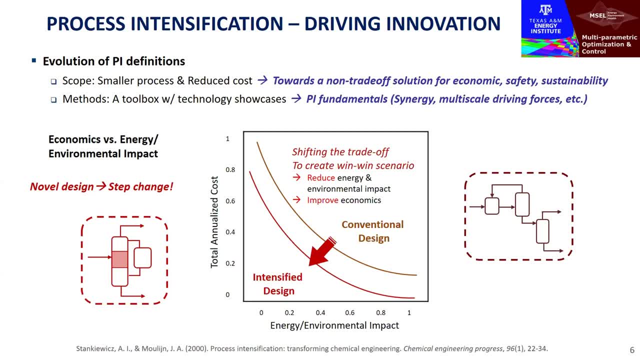 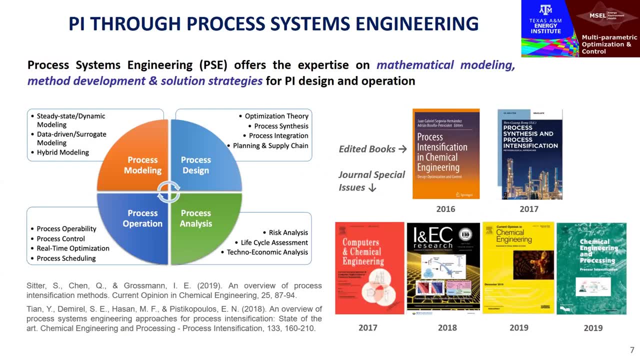 of how this can be achieved in different ways. So essentially, you know, the process systems engineering community has heavily contributed to this space in terms of mathematical modeling, method development and solution strategies, And there has been an explosion of both edited books, special issues, and you know. 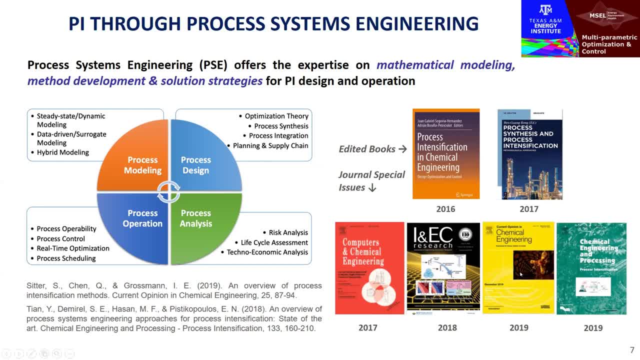 there have been a number of overviews: one by the Professor Garry's group- I'll mention this later on- one from Ignatius' group and one from our own group back in 2018.. And this review paper And this has been receiving a lot of attention, which really signals the importance of processification. 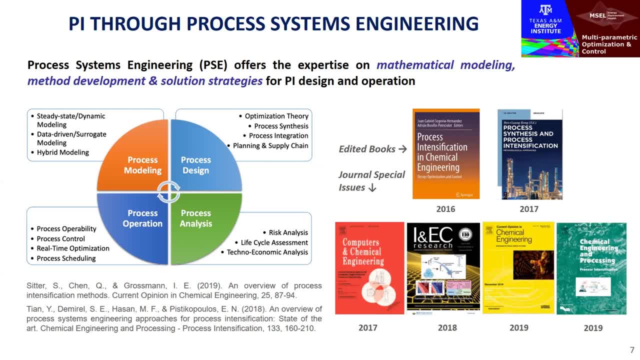 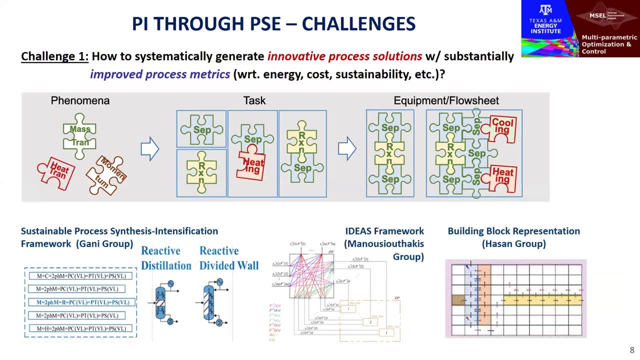 as part of the portfolio driving process innovation. So let's take a little bit more systematic, like looking into the challenges that you know. obviously we all would like to incorporate processification thinking into our development, but what are the fundamentals? 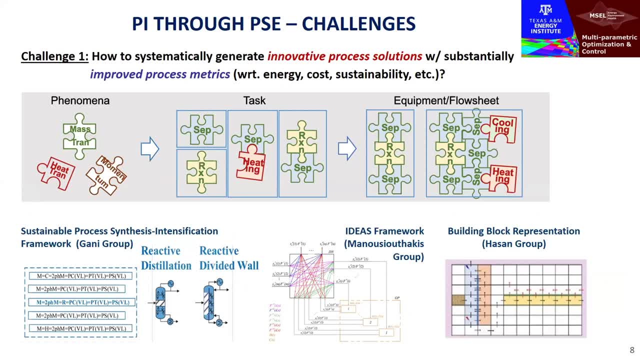 What are the fundamental challenges that we have to overcome, And I think Professor Garry already highlighted that challenge number one is how to systematically generate such intensified solutions which can guide us towards or drive the process system towards improved process metrics with respect to sustainability, cost, energy and the like. 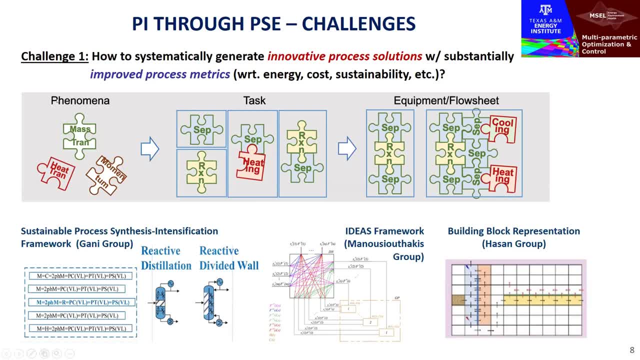 Right And the key, the devil here is environmental, the detail like how can we capture the various phenomena, reclassifying them at us and then try to develop the equipment at the flow sheet? as a result of this- And you know, you have seen already- 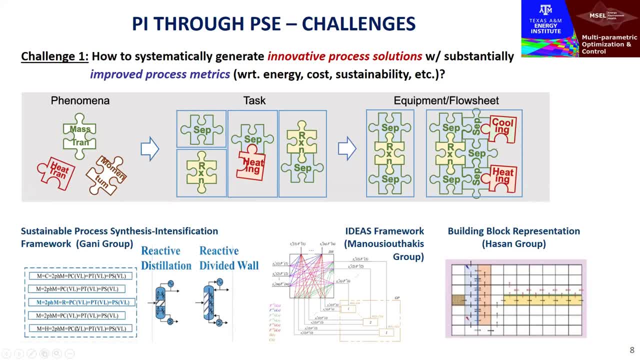 just a few minutes earlier, you know, Rafik was highlighting how you can do this systematically through a representation that takes a systematic procedure, by analyzing your current equipment, transforming this into tasks and then characterize the equipment and then re-synthesize. 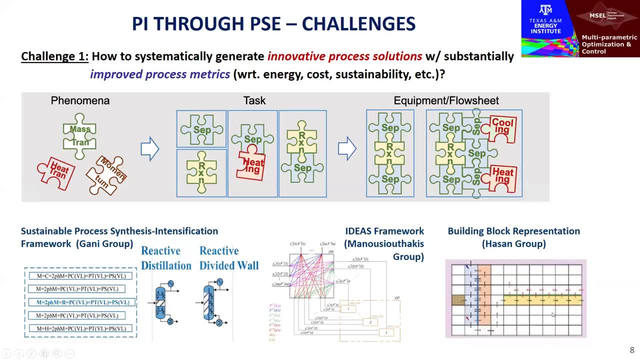 try to combine. There have been other representations as well, based, for instance, there's a building block representation by the group of Farouk Hassan, there's the ideas framework by the group of Professor Manoush Yudhaikis at UCLA, and so forth. We'll come back to the 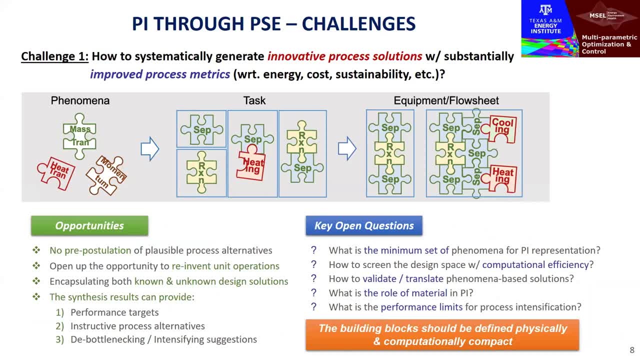 representation. So clearly there are some open questions in doing this, you know. one of the things is: you know how can you do this in a way that you don't have to pre-postulate all possible alternatives? you know. So, essentially, what is the absolute minimum set, a minimal set of phenomena that you 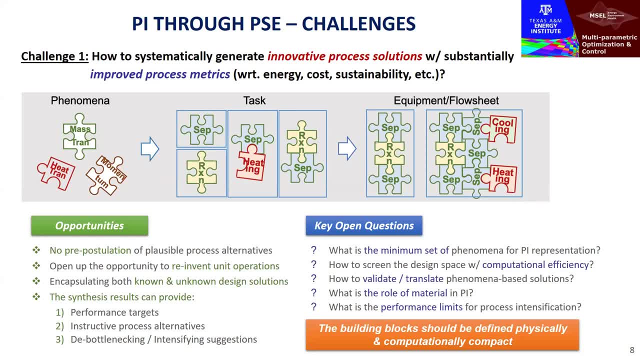 could unlock processification possibilities. How about computational efficiency? You definitely want to avoid that, So you need to find some kind of aggregation, if you will. that avoids exhaustive enumeration of all possible realizations. you know, and then you need to somehow translate the solution you know. 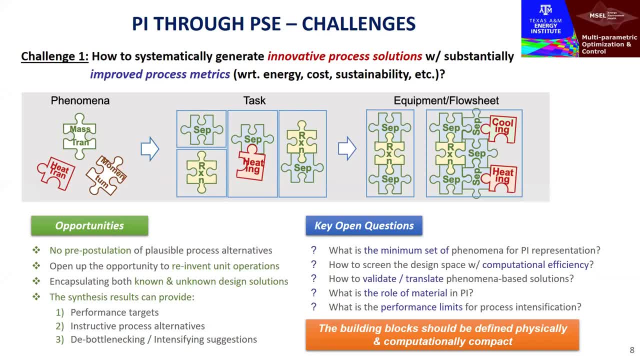 when you're talking about unconventional designs. how can you link this to simulation- things you can do like with standard tools? the role of materials: can we define a priori performance limits which essentially can guide the sets and things like that? So, and the key aspect here is, you know, 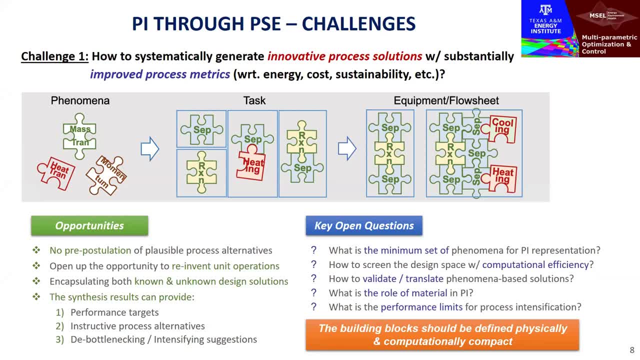 so we need to define building blocks which are both physically and computationally compact, so that we take both the complexity of the representation and of the phenomena that may take place, as well as the resulting computations in terms of a computer-based mode. 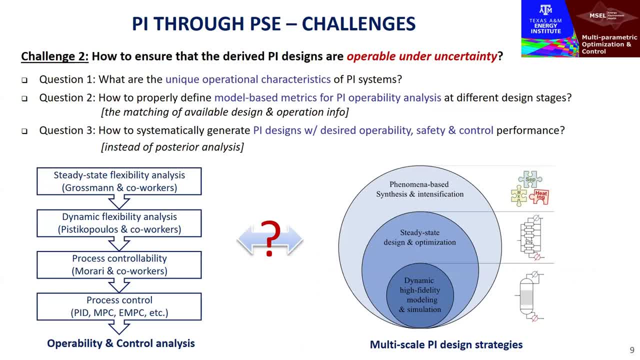 The other major challenge, obviously, is that you know we need to understand, by putting phenomena together, when dealing with uncertainty, disturbances and from a control and operability point of view: are we going towards the right direction and how can we head so that we're? 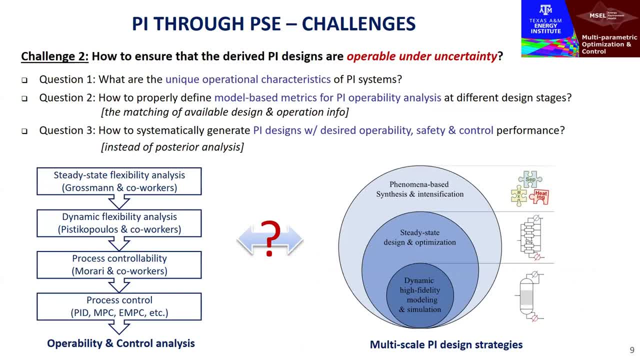 sure that the derived intensified designs indeed possess the operability characteristics that we would like to. So, and we'll talk about this. you know there are a number of questions. we'll come back to this and I will present to you a systematic procedure in tandem with the synthesis framework, which 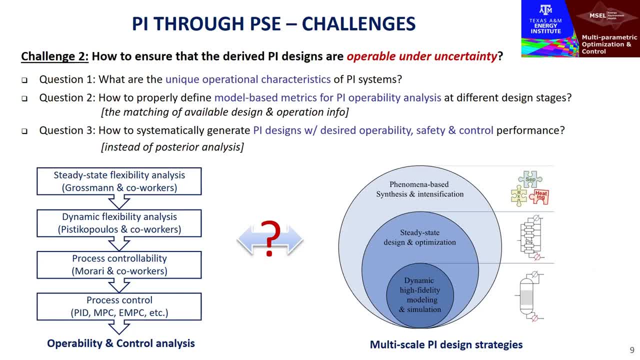 addresses some of those issues, But that's critically important because we need to understand fundamentally by combining phenomena. are you going towards modular designs? do you? what happens to degrees of freedom? what is the role of constraints? because, for instance, you might lose constraints that we can physically 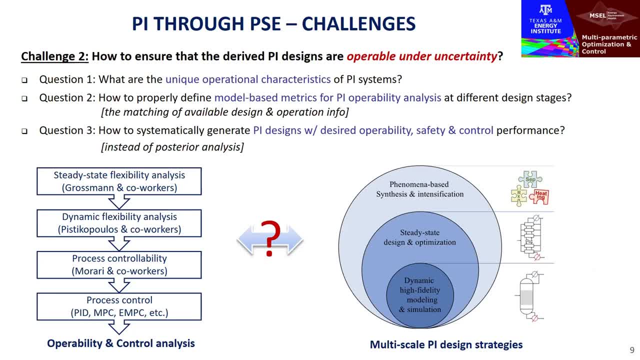 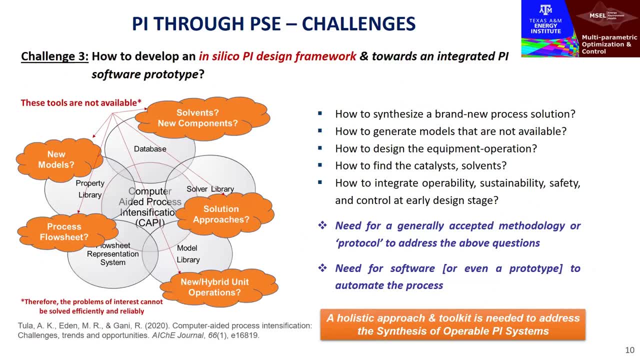 take care of through control if you have non-intensified systems. so we need to understand this space a bit more in depth And finally, obviously, we need to transform all this knowledge into a systematic framework that can be in silico. capture this and we need to build tools that. 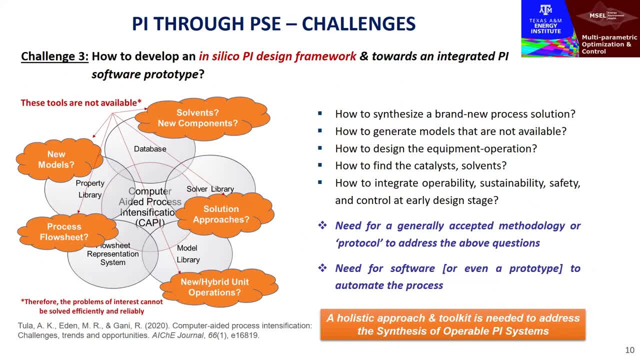 perhaps are going beyond the tools we have here. Here I highlight, on the left-hand side- we have seen this in the context of these webinars- the efforts that have been originating for over 30 years from Professor Ghani's research and right now, under the umbrella of PSC for Speed, we have seen a flurry. 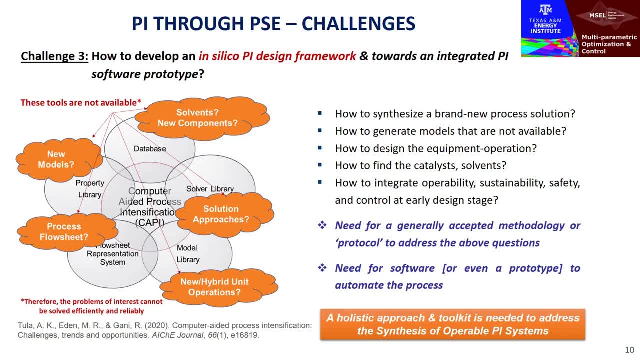 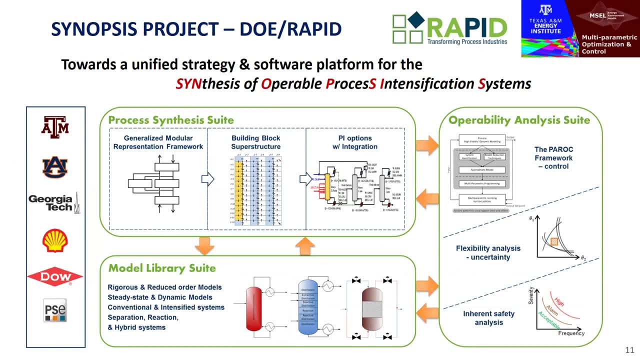 of software components which empower us towards this direction. So let me come back to synopsis and give you a synopsis of what the project is all about. So, as I said, first of all, it involves a consortium of three universities: Georgia Tech, University of Auburn and Texas A&M. 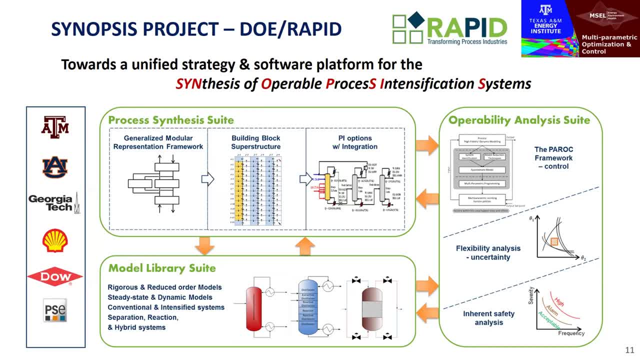 and three companies: two industrial companies like Shell and Dow Chemicals, and one software company, Process Systems Enterprise, now under a Siemens company. So it involves three suites. So we have a process synthesis suite, an operability suite and a process synthesis suite. 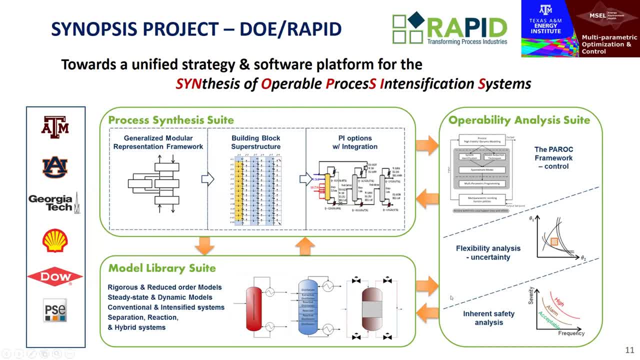 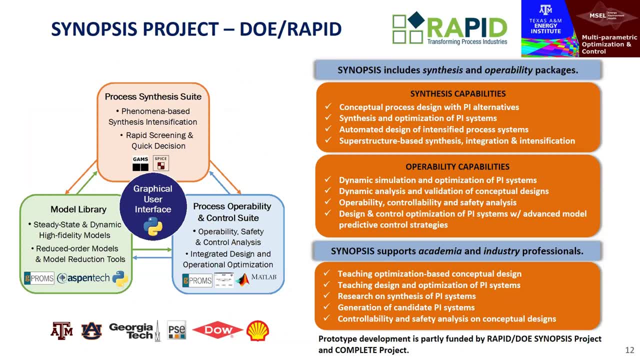 So I'll elaborate a little bit to show you the breadth and depth of this development. So I will also later demonstrate the current status of our prototype software development that encapsulates, or tries to encapsulate, all these components in a systematic manner. All right, so let's backtrack first. 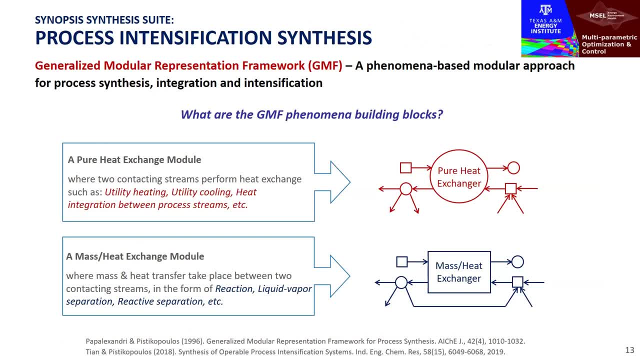 We talked about the need for creating a minimal set of phenomena that can unlock tasks and potential designs to identify matter that is also attractive from a computational point of view. So at the heart of the presentation I'm going to present to you is the so-called generalized 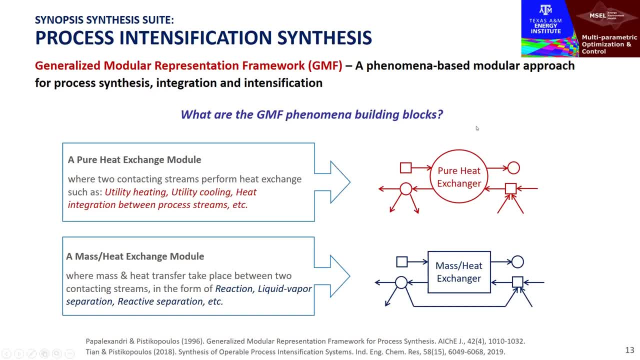 modular representation framework. All right, so this is our building block. So this building block comprises two components: A pure heat exchange module, where you can visualize this as two contacting streams and can represent a utility heating, a utility cooling, a heat integration between process streams, etc. And the mass heat exchange model, where there is a 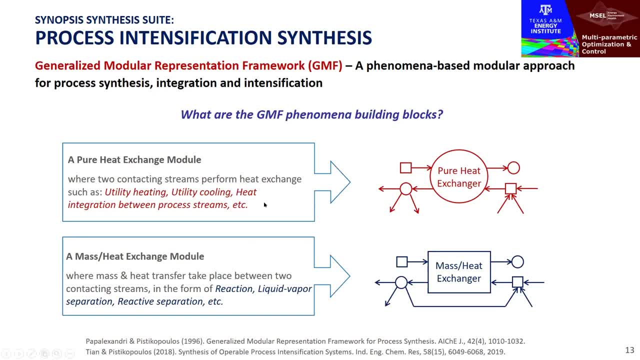 massive heat transfer taking place between two contacting streams, which can be in the form of: in the moment of reaction, liquid vapor separation, reactive separation and the like. So these are the foundations of this framework. So we have been working on this for the last. 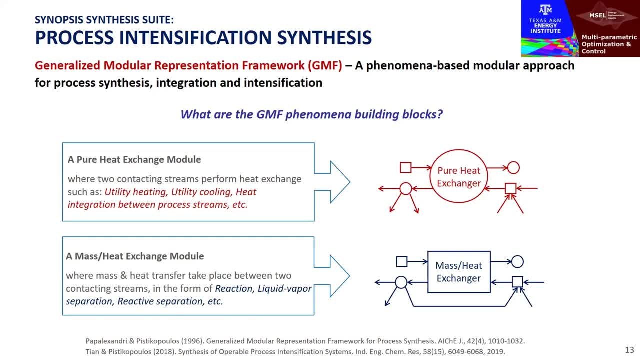 I mean- I'm not very good in subtraction- but at least 25 years, So it's been something that you know. actually we have- and this is part of many developments over the years at the Imperial College- through many collaborations with European Union projects- that where both Rafik and I have been. 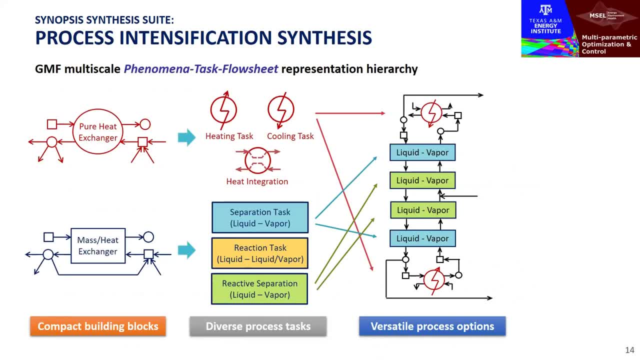 participating, and recently here at Texas A&M. So let me focus a little bit on the importance of representation. So here on the left-hand side, you see these fundamental building blocks. We'll see how they are empowered in a moment, So you can visualize this as that. So this is now a 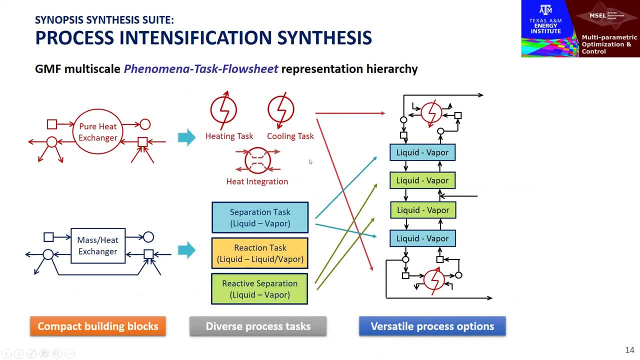 building block that keeps representing various process tasks in a multi-purpose way. So it can be a heating task, a cooling task, a heat integration, So you don't have to pre-postulate the exact task characteristic a priori. Similarly, the mass heat exchange building block can correspond to: 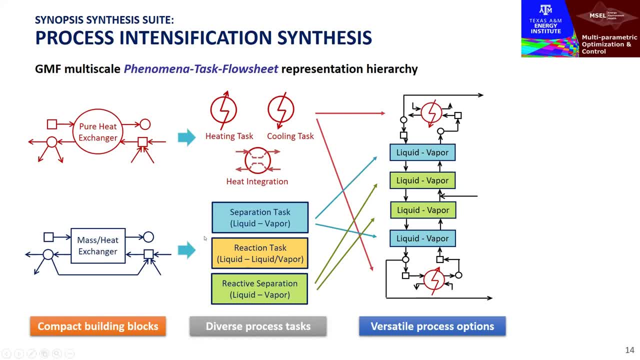 a diverse portfolio of process tasks, like separation tasks, a reaction task, a reaction separation. So again, the mass heat exchange building block can be a multi-purpose way. So again, without having to pre-postulate, And then by doing this, by putting those tasks together, 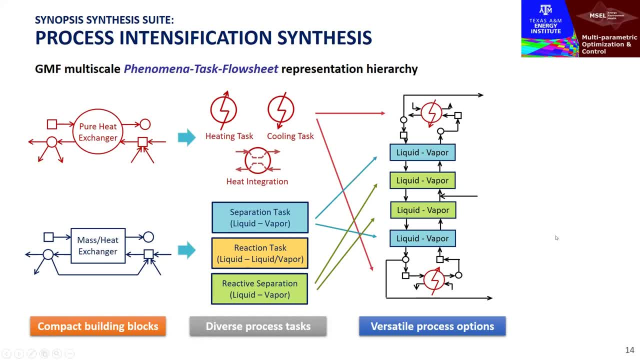 you can start deriving versatile process options, right. So that's the idea. So putting those building blocks together and, for instance, and then you can start addressing questions, how to identify these different tasks from a single phenomena-based module. So this is at the heart. 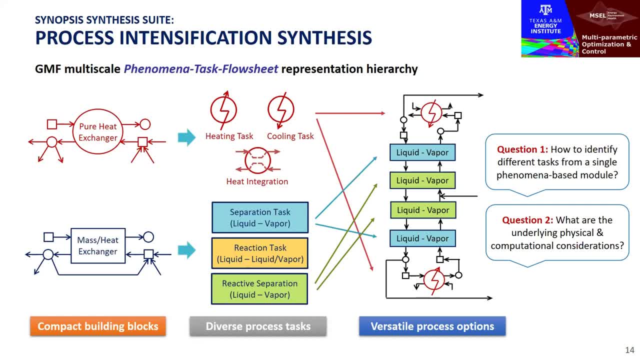 of the presentation. And then what is the impact of this in terms of computational complexity? Because we don't want to solve very large scale optimization problems, obviously neither to simulate infinite possibilities, So we'd like to tame also the computational complexity as much as possible And that offers this possibility. 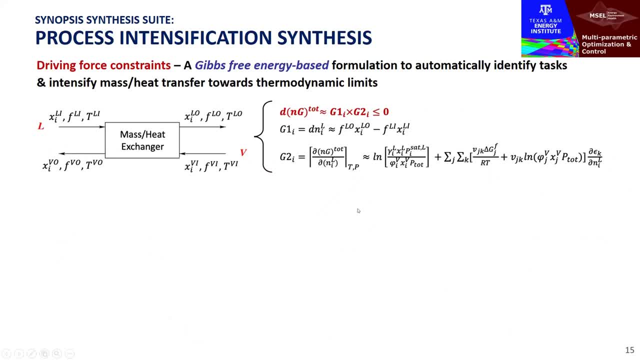 So let me give you a little bit of the gist of what is behind this representation. It's that this drive is the driving force. constraints constitute the backbone, the heart of the ways of the presentation, And it gives free, energy-based representation that allows us to identify tasks. 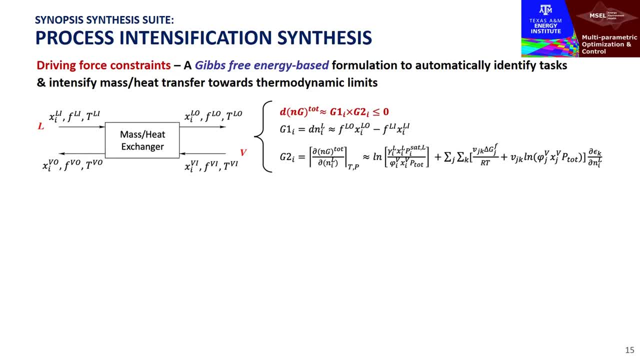 and intensify as appropriate, mass heat transfer by driving the system towards, not exactly to the thermodynamic limit, but towards the thermodynamic limit. So if we take a look exactly how this principle works, so for the mass heat exchanger of this one. so this is the 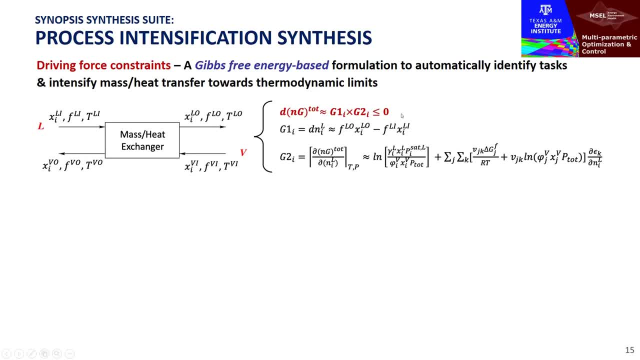 liquid side. this is the vapor side. essentially, you know the system, you know, in order for anything to happen, should be going towards the direction of the minimization of Gibbs. free energy And you can see now a propellant component. so that involves two terms: one that dictates, 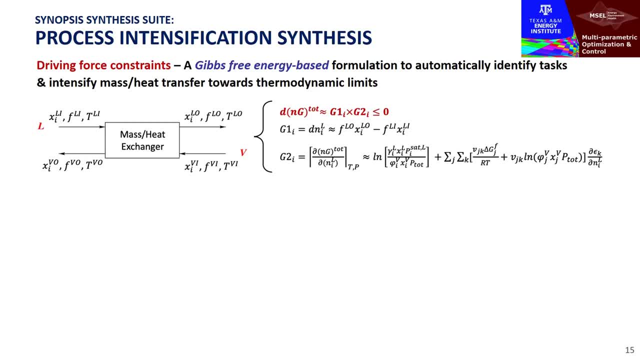 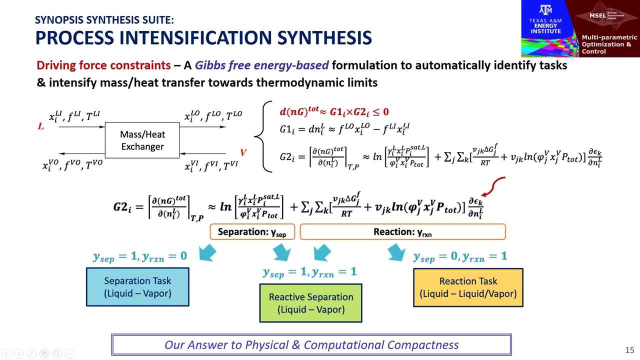 the transfer of material from the system to the system and the other one that dictates the transfer of material from the system to the system. So that is the one side to the other, and then the more involved, if you wish, term that stands for various factors. for instance, the first term here stands for the separation. 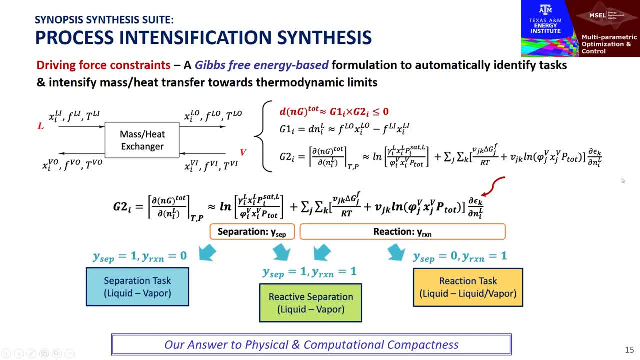 is primarily due to the separation and this term over here is due to the reaction. And now you can visualize. because of this richness of the representation, then, by a judiciously selected and guiding the search through the use of auxiliary zero-one variables, you can activate. 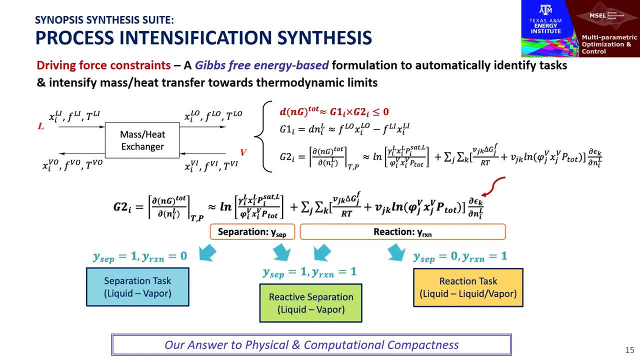 or deactivate various terms in this driving force constraint. For instance, if the second term here is deactivated and only the first term is activated here, then that corresponds to a separation task. If, on the other hand, that term does not exist and only this, 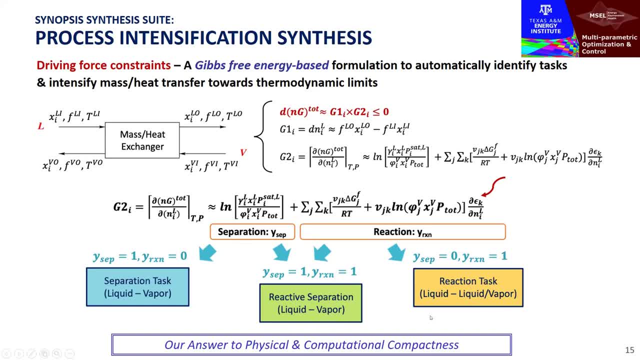 this term exists, that corresponds to the other limit to the reaction task, and if both of those quantities are playing a role in the system, then this can be realized as a reactive separation system And that offers concrete evidence and possibilities for physical and computational compactness. 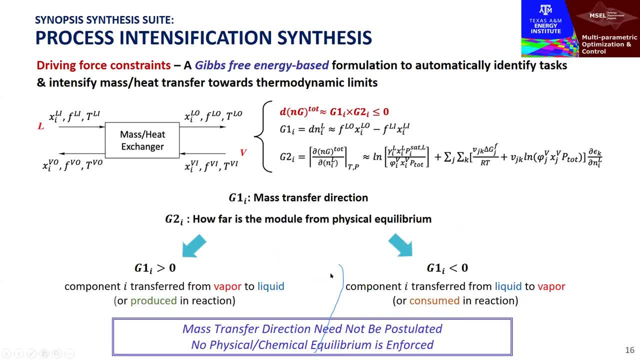 as we're going to see in a moment. So what is this? An artistic? it does not, you know. so now, the key also here is to understand that you know this first term dictates if you use the mass transfer direction. the other term 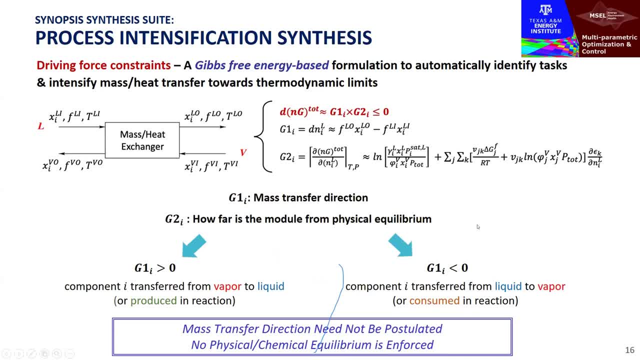 is how far you are from physical equilibrium. We don't enforce equilibrium. So therefore, first of all, you know, you can see that if you concentrate on the first term, if it is possible, we don't even pre-concentrate. 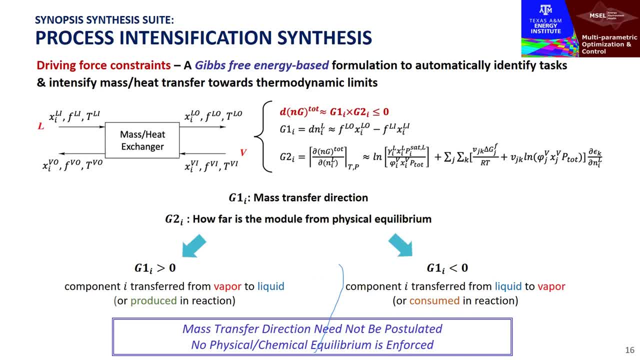 If you postulate the direction of the mass transfer, this is also dictated as a result of the analysis. That's another key power of the aggregation. So if this is positive, then that implies that you have a transfer from the vapor phase to the liquid. or if you extrapolate to the reaction that is produced in the reaction, 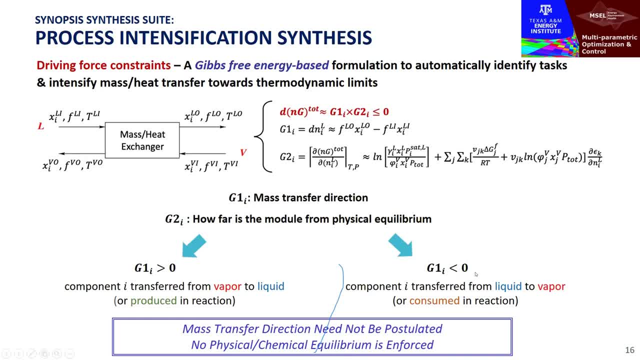 If that term is negative, that means the component is transferred from the liquid to vapor or consuming the reaction. So therefore the mass transfer direction doesn't need to be pre-postulated, And also we don't enforce a priori neither physical nor chemical equilibrium. 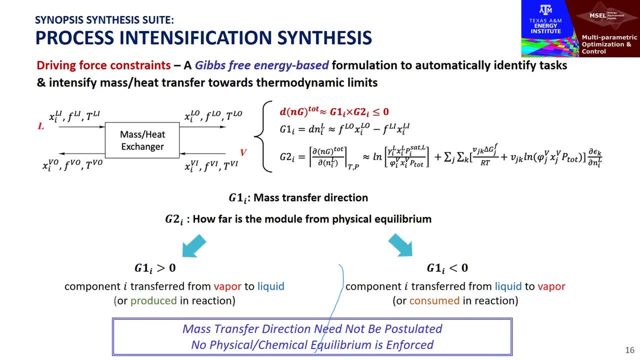 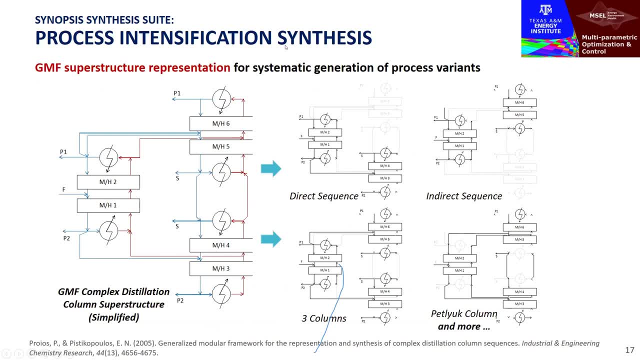 We let the system go towards the direction that makes this the most attractive option. So, and let's also, from a compactness point of view, just I want you to highlight, for instance, the power of the representation. So here is, let's say, pre-postulated, you know, by putting these building blocks together. 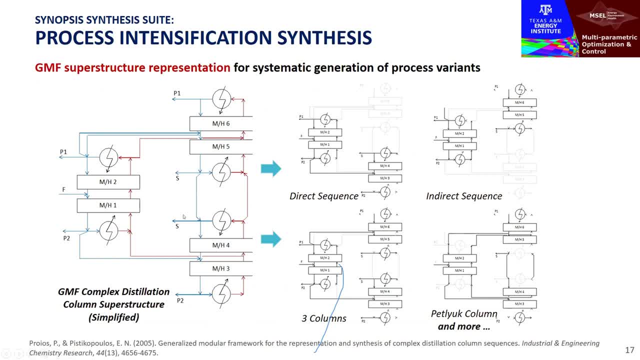 in the context of the so-called superstructure. let's say, you put six of those modular mass heat transfer and you put one, two, three, four, five of the heat components and then by just simulation you can see this. 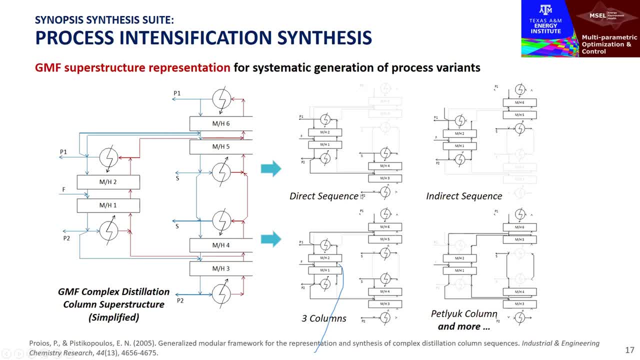 So you can see this, You can see this, You can see that we can unlock the direct sequence here, the indirect sequence here, the three-column configuration here, the petal column here, and so forth, and so on. right Again, without pre-postulating. 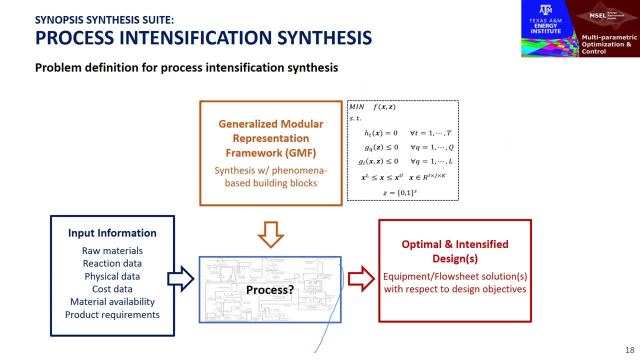 So just simply by simulation, All right. So how do you put this in a synthesis context? obviously, here we try to solve. you know, we pose this as an optimization problem, obviously. So you have like input some characteristics. 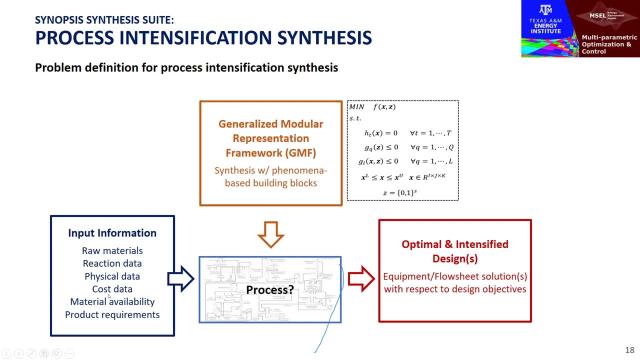 So you have, like input, some characteristics, Some parameters, like what type of raw materials, the oxidized, anything that needs to be provided, the product requirements and so forth. Then you are trying to achieve an optimal design which includes the intensification. 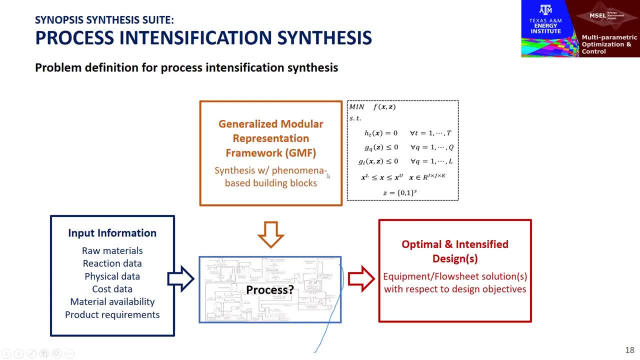 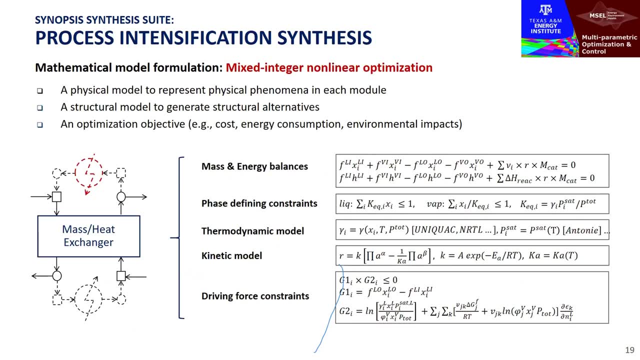 options, And then you build the model of the digitalized modular representation and you pose it as a large, as a mix, as a nonlinear optimization point. So if we look exactly at what is happening in the model you have like, So if you put, let's say you pre-postulate, let's say five, six of those you know you, 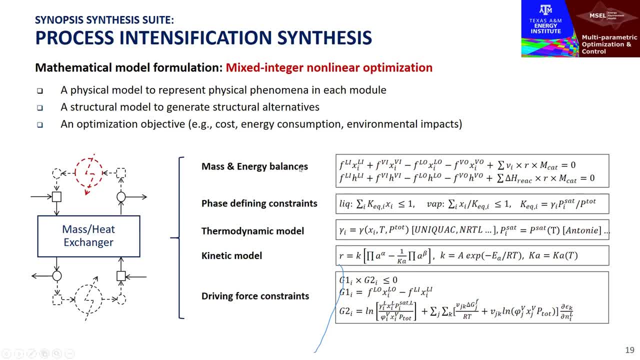 have an upper bound of how many. You only pre-postulate those, nothing else. And then you write the mass energy balances associated with this building block, the phase defining constraints based on the input- thermodynamic models, kinetic models- and then the drive. the key, the heart of the representation is this driving force property. 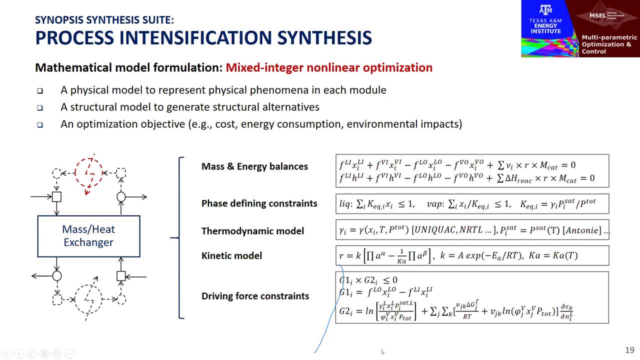 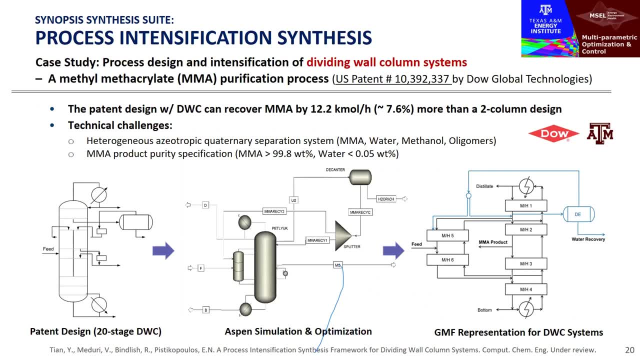 right, Right constraints that I just highlighted earlier, right. So you put those together and the solution comes up with different options. So let me go through an example that highlights the power of the representation in the context of a divisible column. So this is a joint collaboration with Dow Chemicals. 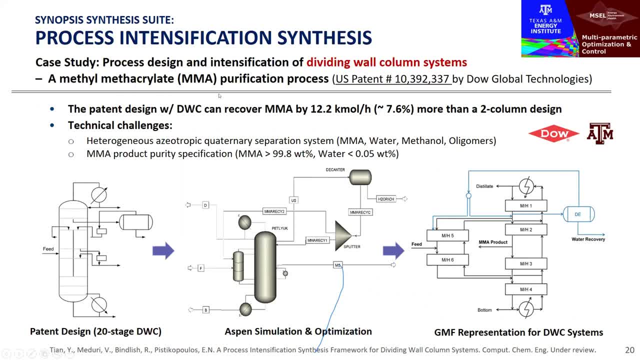 This involves the methyl methacrylate process, purification process, a US patent. and here we saw the US patent involving a 20-stage divided work column right. And this is an aspirin simulation of the system. So to achieve this type of purity specifications- 99.8%, and with less than 0.5% in weight of. 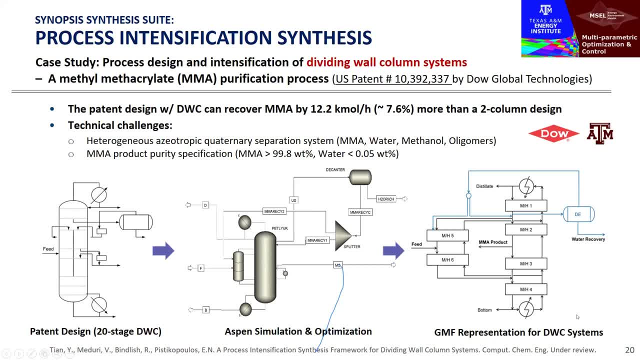 water, And this is the combative process. Okay, So that's the representation of this equivalent system based on the generalized modular framework, And you know so it suffices with only six modular heat modules and two pure heat modules. You represent exactly the system. 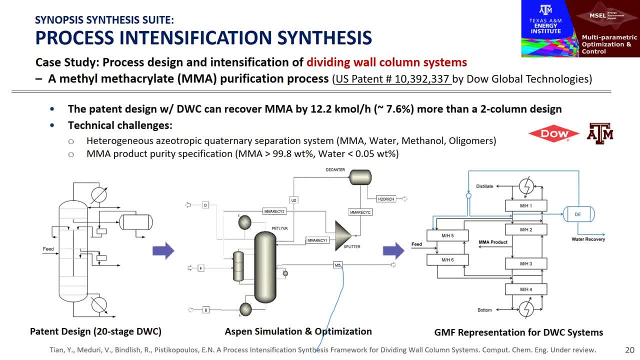 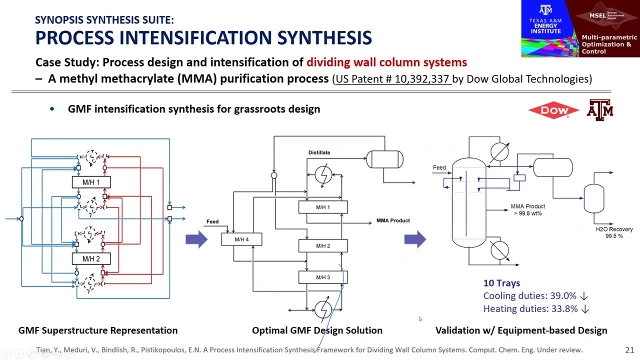 And this can be viewed as a starting point for doing the stuff right. And here so again. So this essentially reproduces what the patent is all about. Now the question is: can we do better than this? So one way to address this is to do like a grassroots design. 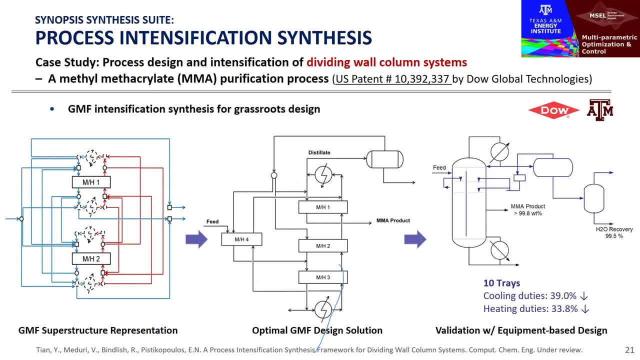 So not only proof what we hear. but if you had to start from a, from a clear set of paper, how would you do So? here we postulate a number of those modules together, and this is the structure that we come from. 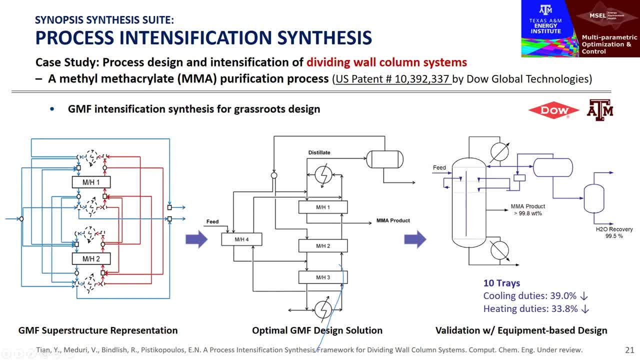 we postulate here- up to 10 modules. This is the result: It picks four of those modules and two pure heat modules, And then we translate. I will show you in a moment how we do this. we translate this into an actual simulation which corresponds to this divine work column with 10 trays. 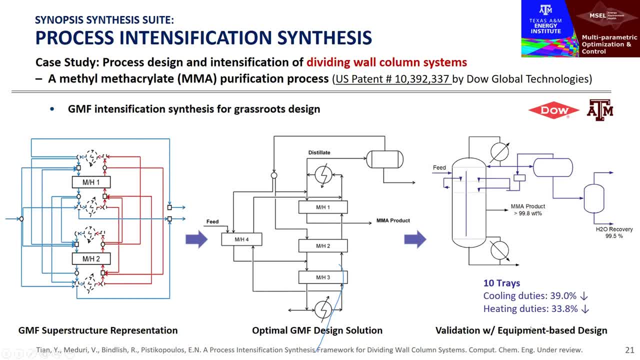 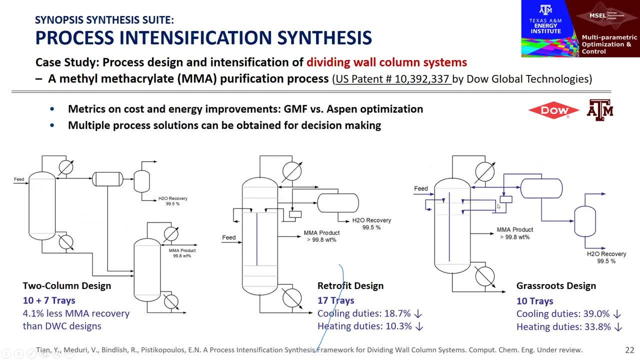 And you can see that the derived design now has drastic improvements, you know, compared to the initial part of the design in terms of the heating and cooling. So this is a validated design And you can actually ask the question: how about? so here you see like three. 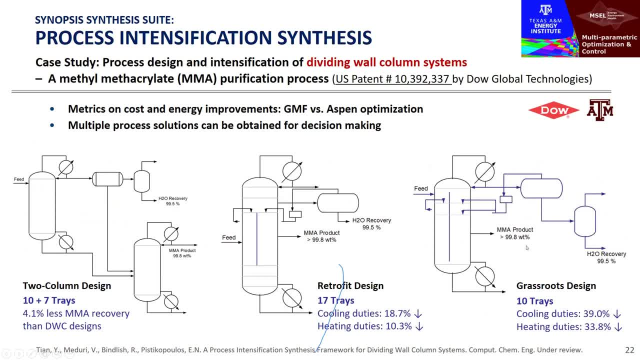 designs that we obtained from the result of this type of representation. So this is the gradual design which has been validated through also the representation. This is the retrophic design. So if we start from this and we're trying to improve, it is the 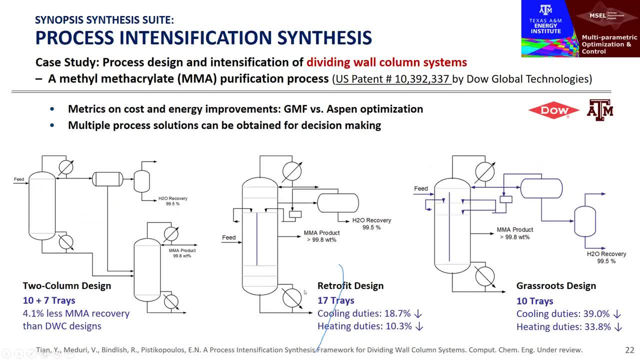 you know what I showed you with the improvements in terms of, corresponds to 17 trays and with, again, not as much improvements but still significant, And this is the two column design. So this is the non-intensified system Which can achieve, you know, close to the pattern but not with. perhaps it doesn't meet quite. 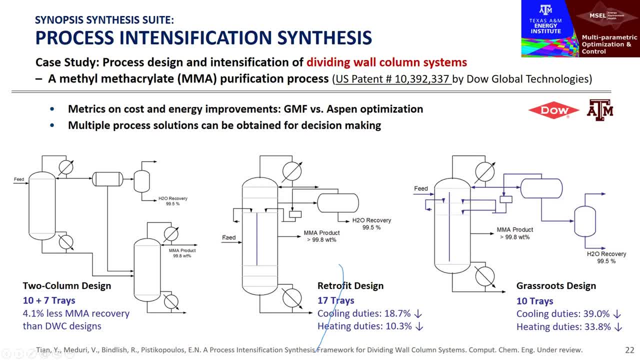 the recovery specifications, but so perhaps it needs an extra unit or so forth. So, but from a citizen's point of view, you know, the key message here is that we managed to unravel for a very compact representation, not only represent exactly the pattern, but unravel three extra designs. 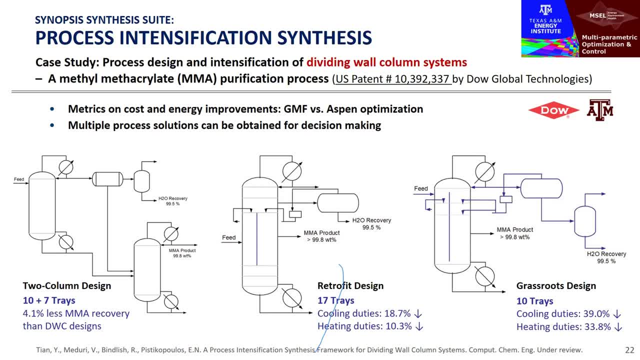 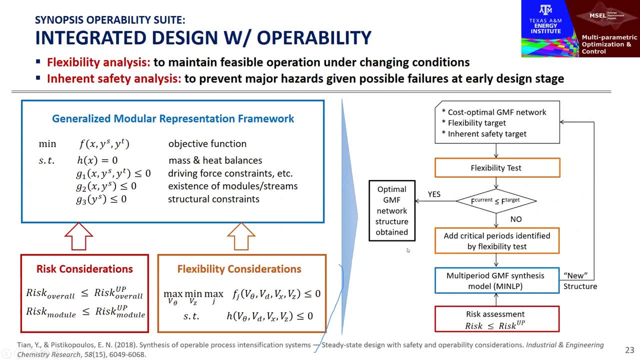 for which can be further studied and validated. So all right, So okay. So those are now designs. but you know, I mean obviously you need to ask yourself in these designs now how they can perform in terms of operability. you know, can they operate physically under changing? 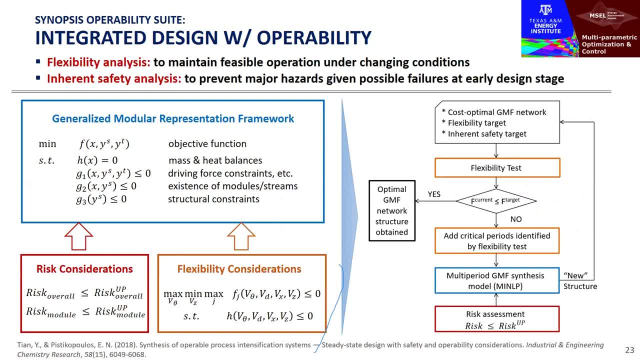 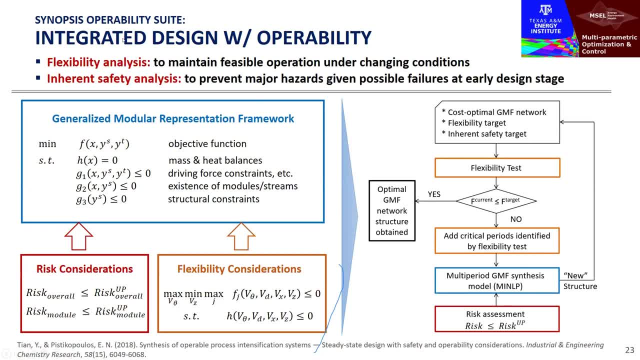 safety or not, you know So. so accent the presentation. This exactly what the legislation. you're ready to go earlier and we start. we have a way to incorporate flexibility considerations. There is rules of Arc science's safety defense and approach that essentially involves and iterative procedure of the muitolevise designs. 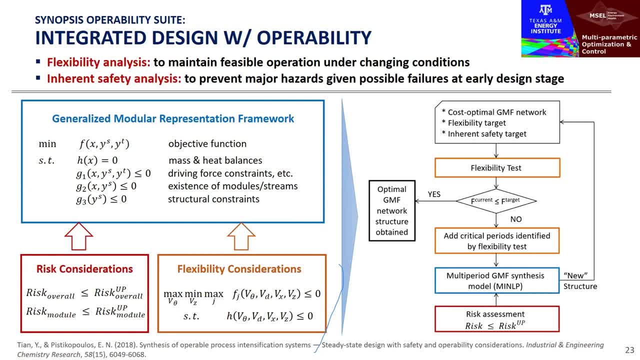 taking tissue. that is part of the traditional training, where the chasing, Assassin relaison and vis-a-vis flexibility and risk assessment and then taking on board some critical parameters, incorporate them in the design and keep on going until you get a validated structure that also delivers the desired degree of operability. 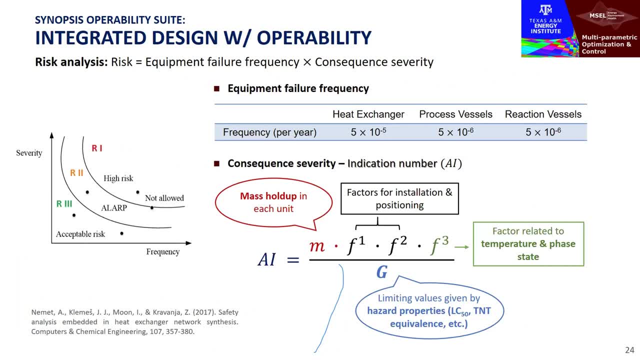 Just as far as risk, for instance, you can use various risk factors. Here is the one we have currently implemented in our procedure. It's a combination of equipment failure frequency and the consequences of disability. So we're trying to see. I mean, the key thing here is we want to see whether the incorporation of flexibility 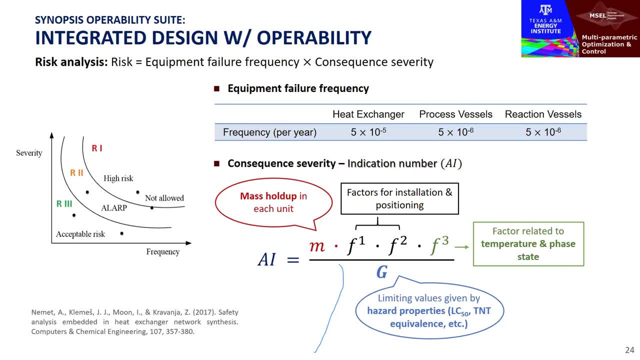 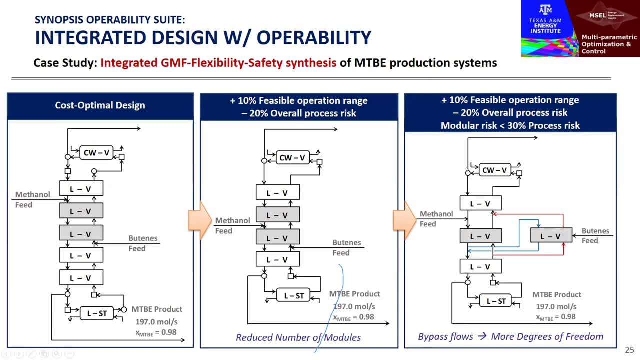 and the risk metrics can change the derived structure. That's what we are after, And here's an example of the MTP production system. So you can see there, This is the evolution of the design, the intensified design. This corresponds to a reactive separation. 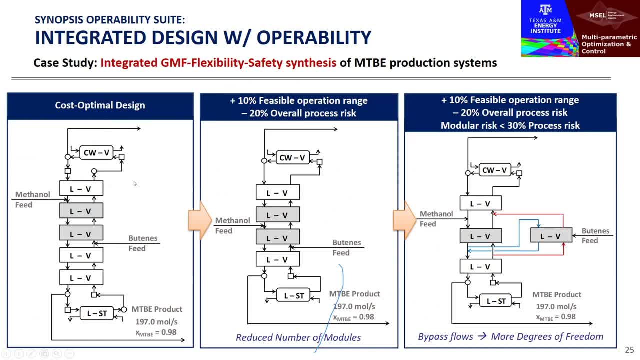 That is the best you can achieve without any operability considerations. So you can see that there are two reactive modules, three non-reactive modules and three pure heat modules, And then, as you increase, as you impose flexibility and risk factors, the design is intensified by reducing the number of modules, further intensified. 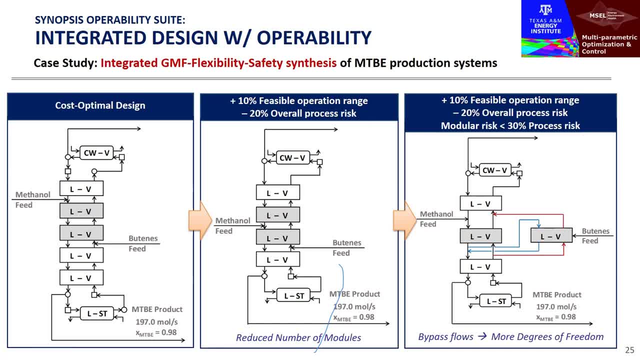 That makes sense from a risk point of view because you know you try to minimize, if you wish, the volume And you can view this as sort of pseudo volumes. But then as you increase your risk requirements towards inherent safety, then the system goes towards an increase of the degrees of freedom. 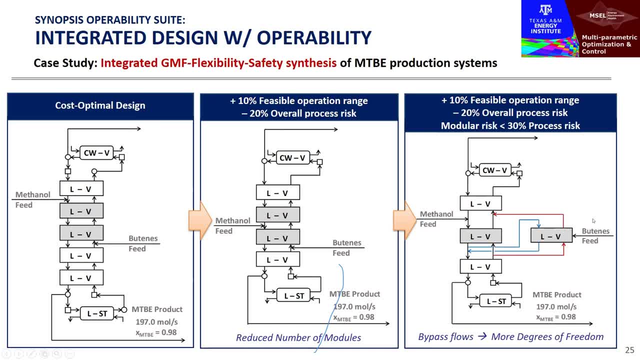 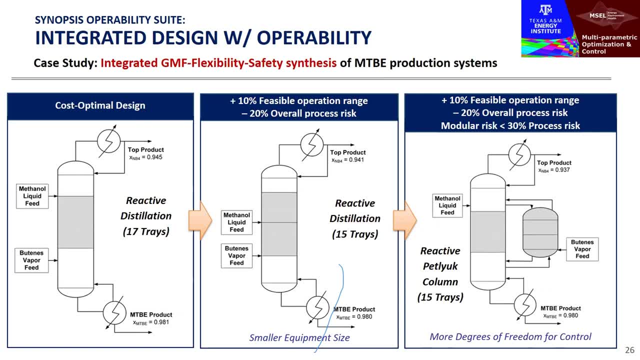 So this makes sense. So it picks a second column and then you can go and validate it. So here are now the resulting posterior systems that you can simulate, for instance through ASPECT, and verify through studies, also through dynamic simulations, that this is indicated. 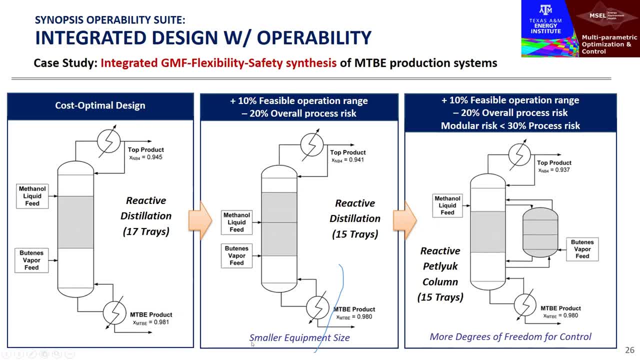 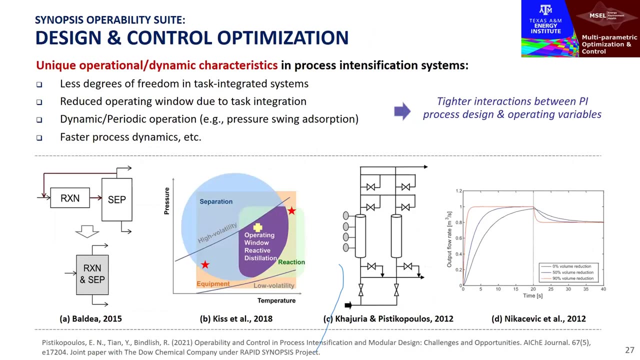 The key point here is that operability is a critical component of a synthesis framework like this. And here you can see, as we introduce operability characteristics, the system understands this and tries to reorganize itself to incorporate and go for to achieve not only an optimal design, but with the desired operability characteristics. 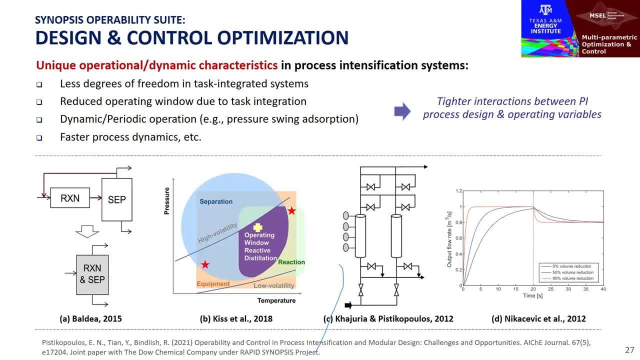 Obviously, that is it We need. also, as I said earlier, you know we need to understand a little bit more in depth, You know, when we're talking about process intensification, what are the inherent properties in terms of dynamic performance of the system? 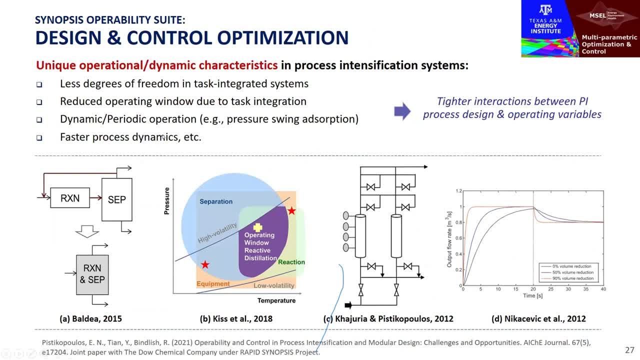 For instance, we get less degrees of freedom, We reduce the operating window, as has been observed by other, obviously, research. that makes perfect sense. You know we have issues related to dynamic periodic conditions, So how we can take this into consideration. 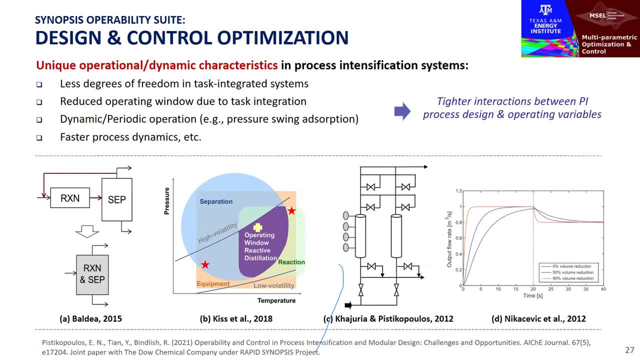 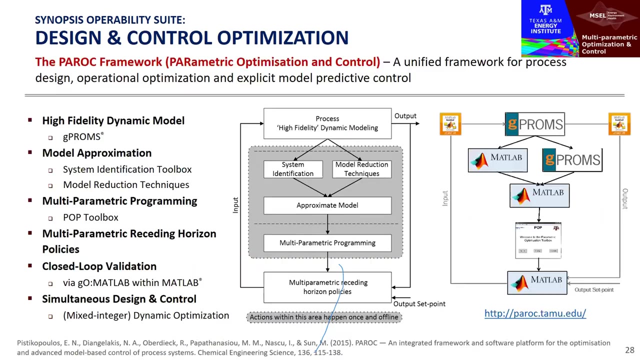 In a systematic way when we aim for process intensification, what about faster process dynamics and so forth? And he works in the open literature that addresses this, And recently we published a paper that talks about a little bit, puts up like a systematic analysis of the various challenges in this way. 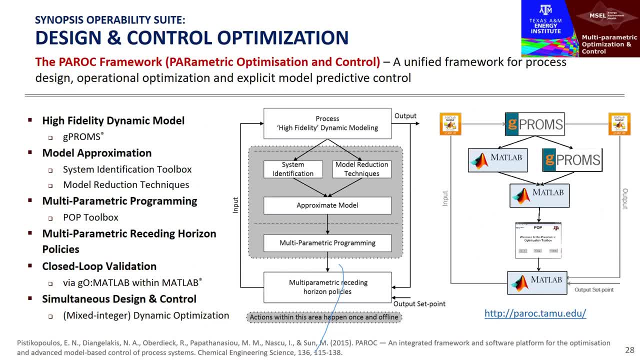 But let me tell you how we also practically deal with this. So now, so at the exit. so up to that point, in the framework we talked about steady state, if you wish, designs with certain degrees of flexibility and inherent safety. this is not enough. 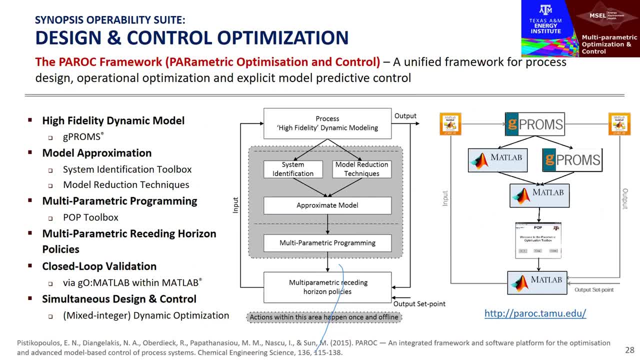 You only test the dynamics, because most often than not, intensified systems fail because of the dynamics. right, You know the dynamic characteristics. So how we do this systematically, then we transform the steady state model into a dynamic model. Usually we do this based on the GPROMS platform. 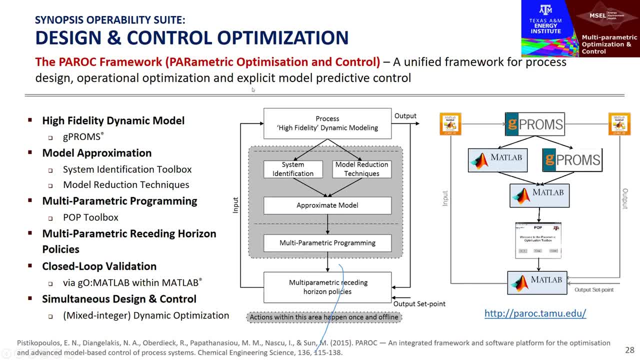 Then we follow the so-called PAROC framework that we have been developing for the last 30 years, that sense of the parametric optimization and control that involves taking high fidelity models, approximate it through certain model reduction system identification techniques, then apply our parametric optimization toolbox, derive model predictive. 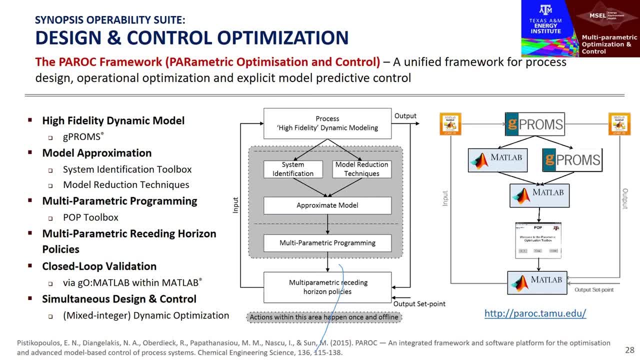 controllers, incorporate those into the model that you started before. So validate in silico the dynamic performance of the system before you embark in this, and offer certificates of guarantee that the intensified system has these operability characteristics and the control system to, along with the design. 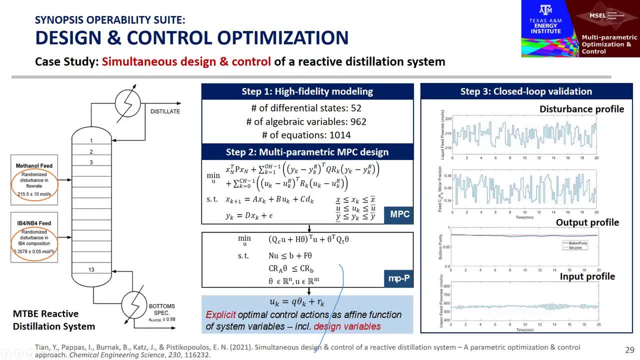 So let me show you how this can be done. So, for instance, here is the way for the MTB system to be studied. You can see here we have disturbances for the inputs on the feed. So you build the high fidelity model. Then you derive an instance which is a system identification, from which 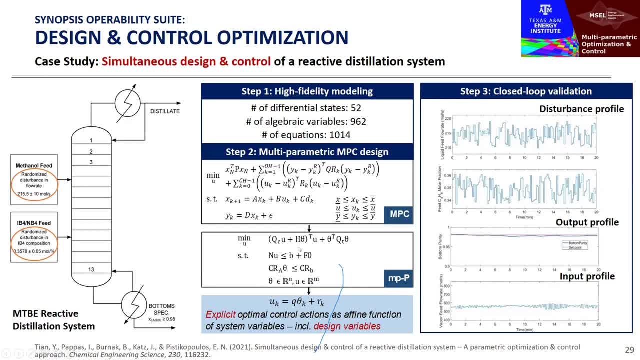 you derive the parametric controllers, You incorporate the expressions. These are the controllers. You incorporate them into the high fidelity model, And then here is a closer validation. So now this is the validated that the reactive separation can really do what is supposed to be doing on the box under dynamic conditions. 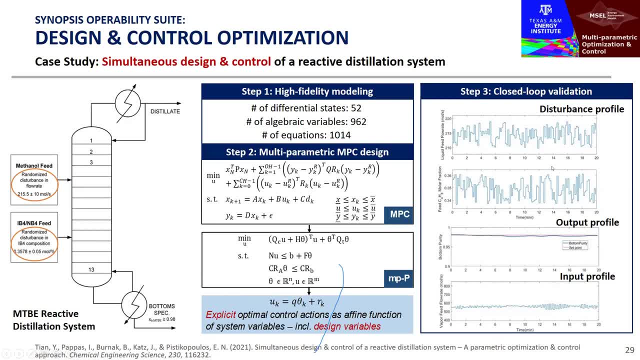 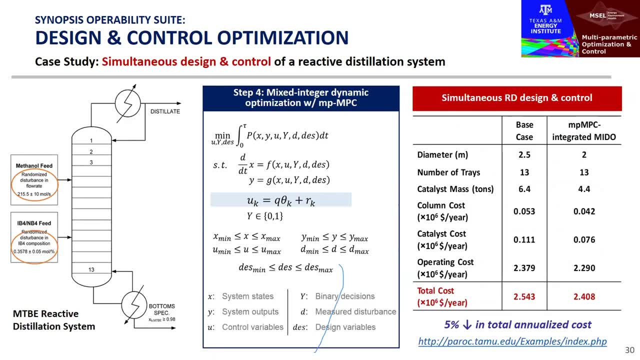 So you don't need to go and do any post simulation. This is a dynamic optimization of the entire system And you can go a step further and do a simultaneous design and control through again by incorporating the explicit validation of these controllers into this design framework. 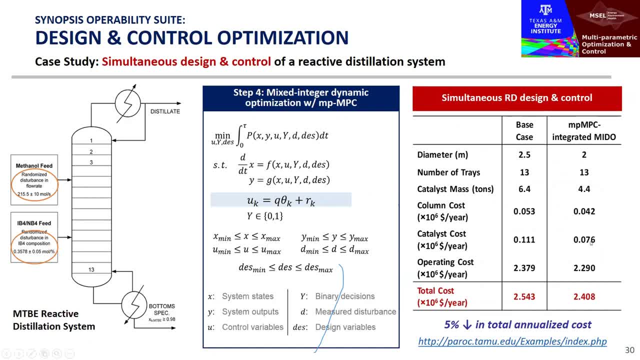 And here you can see this is the base case we started from And this is the case where we have the integrated system with the moderative controller, And you can see that we can- despite the fact this is initially thought to be the best you can- achieve this integration of control and design. 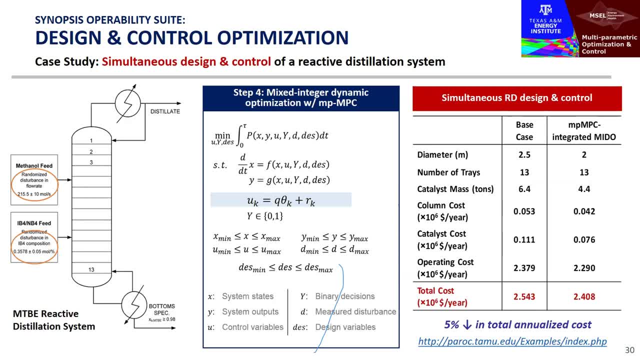 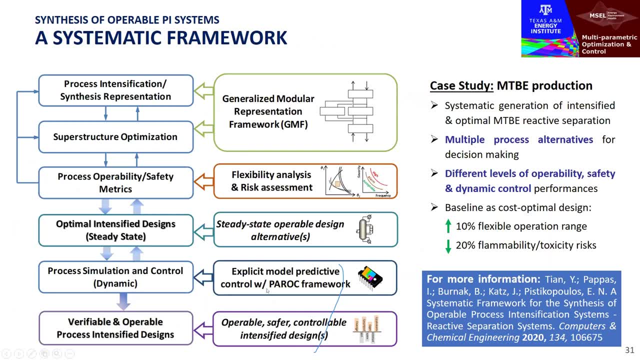 achieves even further improvements. So I highlight to you, if you wish, a systematic framework from process identification based on the rapid, you know the synopsis project where, just to recap what we have seen, we have seen a very compact representation with a minimal set. 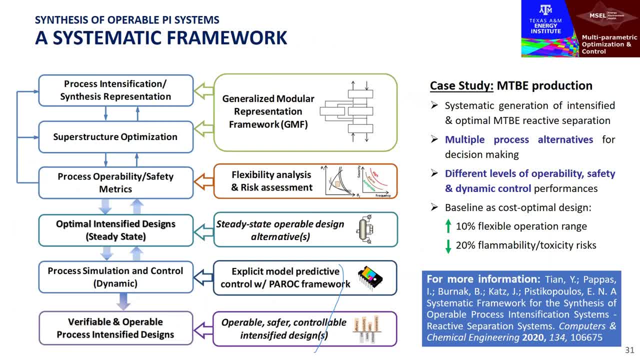 of building blocks which have a very versatile correspondence to tasks and from which you can Generate multiple of processification of computational designs. that reduces significantly the need, the computational complexity that usually one is faced at the support structure level. I have shown you how you go a step further: incorporate at the steady 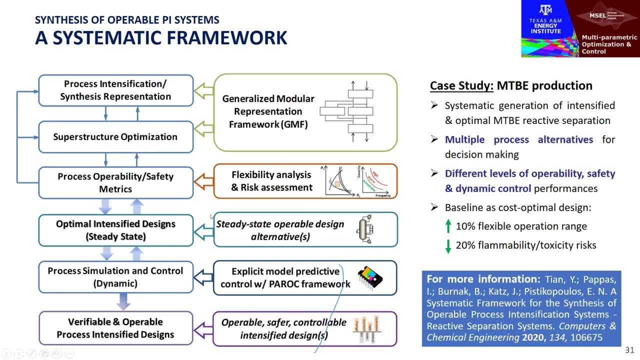 state flexibility and risk assessment considerations. that provides certificates of guarantee from a steady state point of view that the intensified designs are indeed operable. And then one can go all the way to dynamic verification of this through incorporation of explicit moderative control aspects through the PARP framework and then doing a simultaneous design. 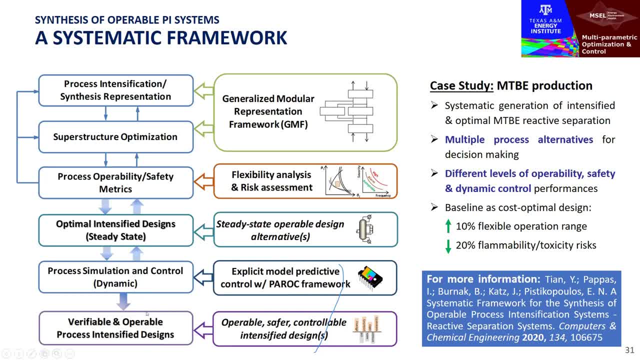 and control. So that step offers verifiable open, process-intensified designs. So closing the loop, if you wish, Both from a steady state and dynamic state as well, And there are some references that I have I will distribute. I will send to Professor Gunn the slides. 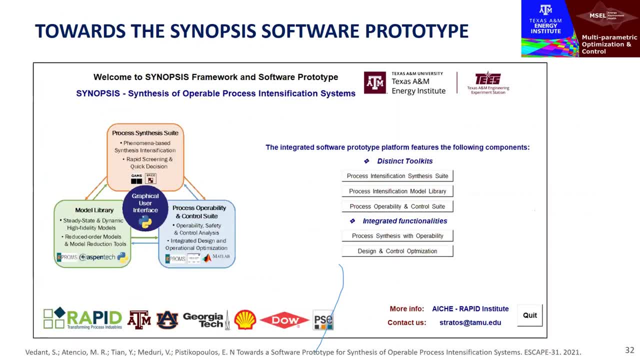 can be distributed to all of you. So this is at a glance. I'll show you in a moment the software. So we have put everything together in a prototype software that we will be releasing through the Rapid Institute towards the September, in fall of 2021. 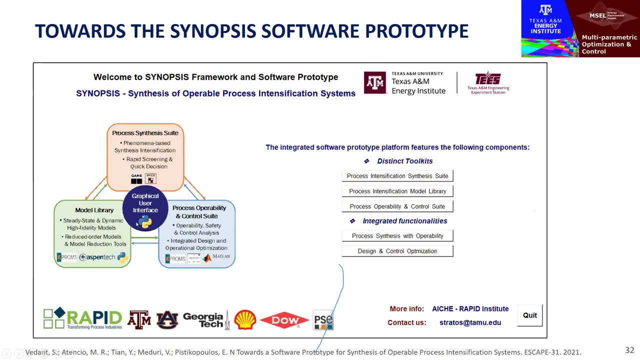 So you can see here that there are the three suites. We have a graphical user interface and there are. it's a toolbox, So it has a number of toolkits. It has the process intensification synthesis suite, the model library, the operability suite and then, in case integrated functionalities. 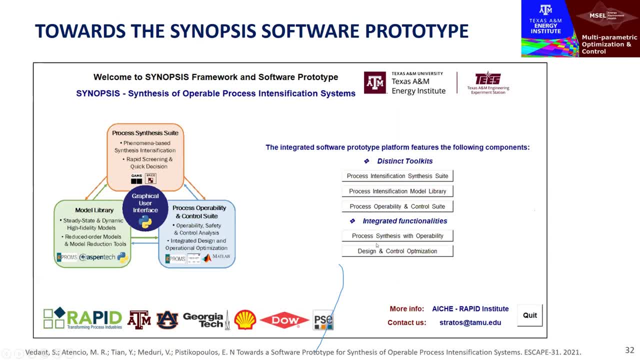 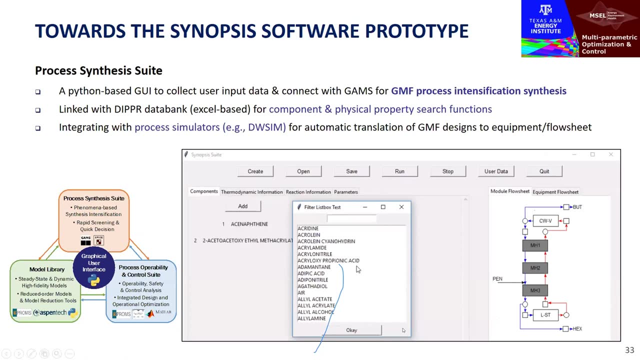 that combine things. For instance, as I highlighted in the exams, you can do the processes with operability. you can do the design and control, optimization and things like that, And we'll see this in a moment. Here are some of the functionalities of the processes suite. 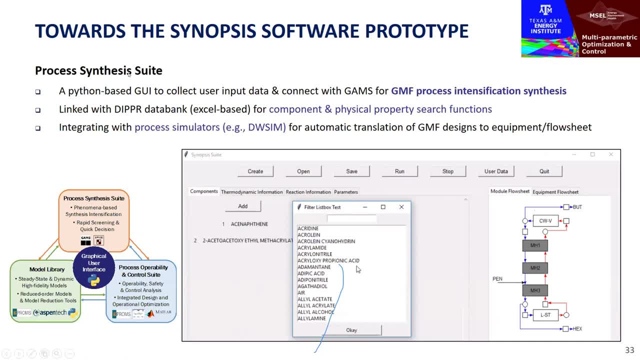 So you can define components. It's a Python-based way that collects input data and connect with GANs. Now we are working on a version that will be everything under Python. It links to various databases, For instance, with the DIPPR data bank. that integrates with processes. 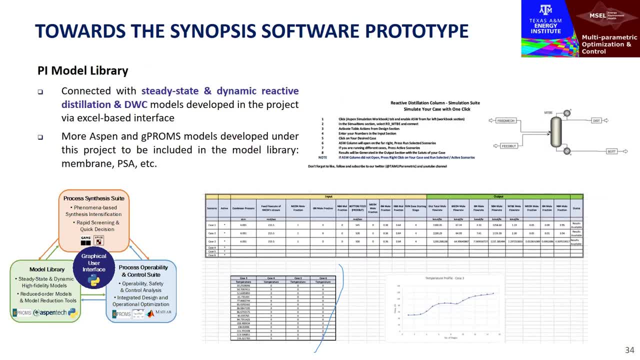 So you can do simulations and so forth and so on. Then you have a model. We are building an extensive model library of validated, stated and dynamically instances for reactive separation, divideable columns, and that will be an expandable set of both in ASPEN. 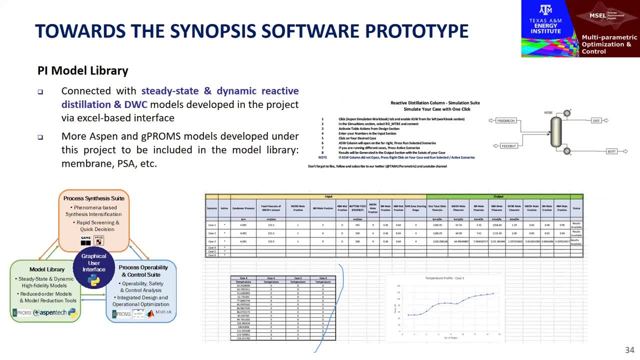 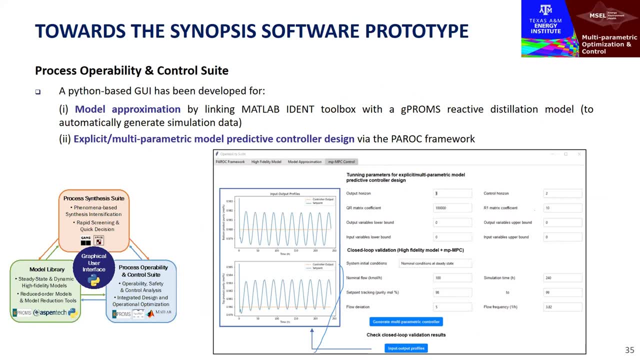 and GPROMs to begin with, And then we have this operability and control suite, which is again a Python-based way that allows us to navigate from GPROMs to MATLAB, to our POP software, bringing back to the validation through an integration of GPROMs and the derived parametric controller. 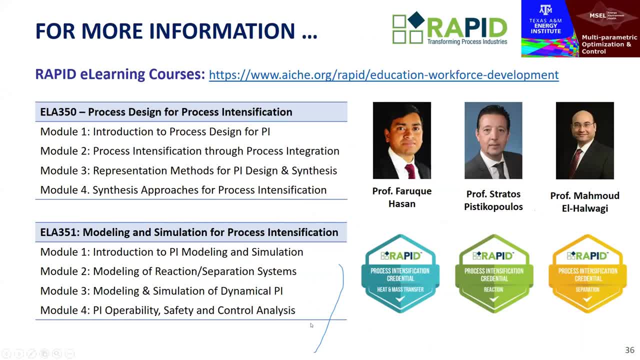 So for more information on this. through the RAPID Institute, we have created e-learning courses, essentially two, along with my colleagues, Professors Hassan and Elkharbaki: one on process design for process intensification and one on modeling and simulation- process intensification. 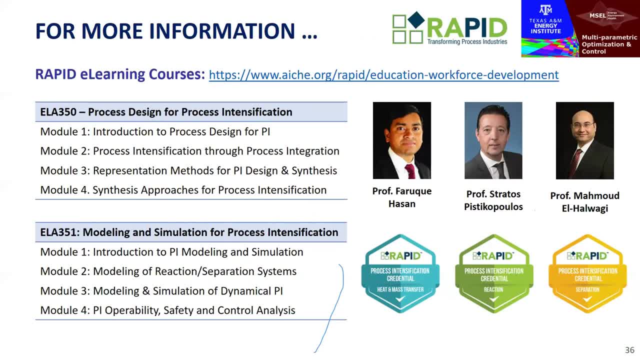 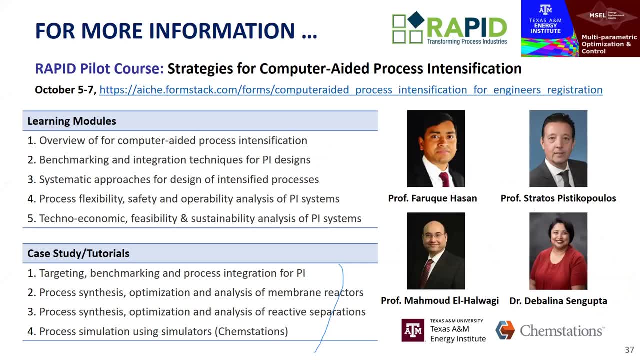 that go through some of the capabilities that I described. but beyond those as well, We have a pilot project, the complete project that we will have under the auspices of RAPID, the pilot course offered in the beginning of the October that involves Texas A&M colleagues as well as chem stations. 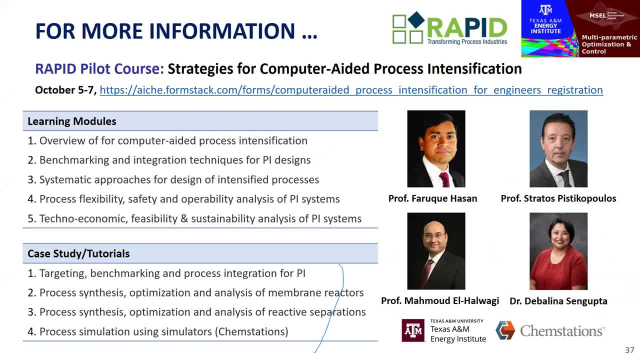 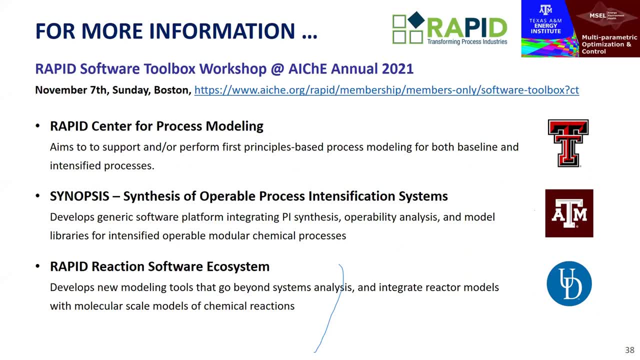 as the simulation supporting the activity company. We're going to have a workshop at the ICH meeting on the Sunday that RAPID is going to run and where you know the synopsis toolbox that I'm going to describe. you know the system, the framework as well as the prototype. 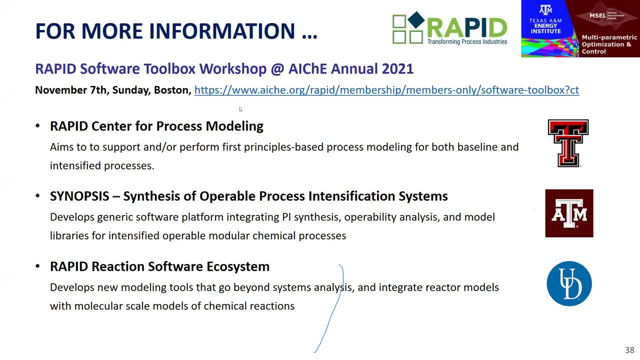 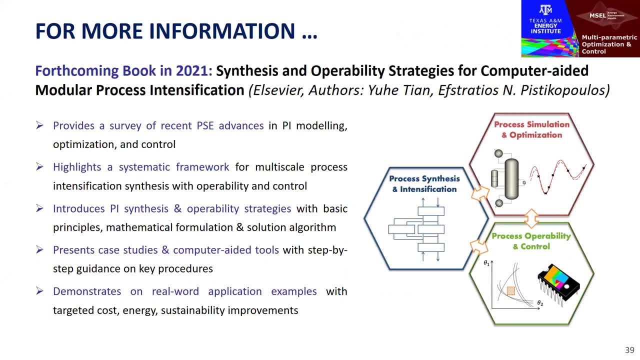 will be presented and along with other tools from other RAPID activities, And there's also a forthcoming book that is going to be out towards the end of 2021 that we are co-authoring. I'm co-authoring together with UKTR. 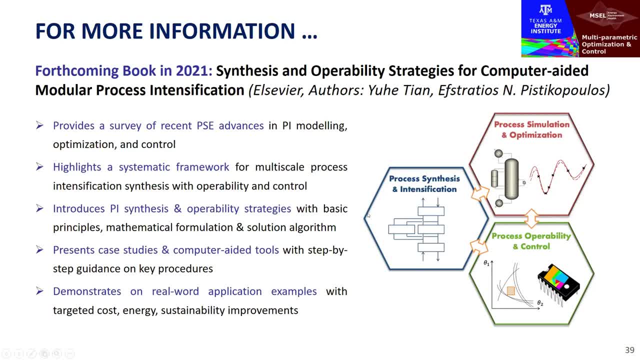 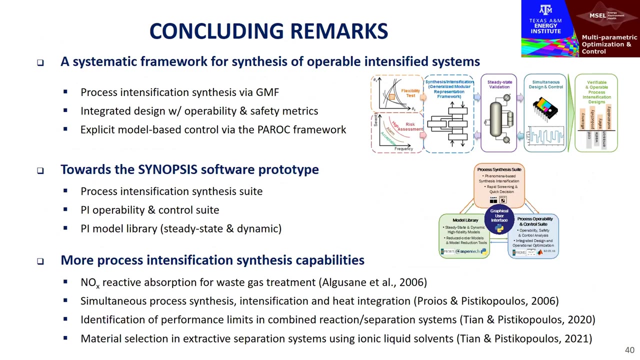 from the University of West Virginia. that will primarily, will be essentially exactly the things that are highlighted. you know, the generalized modular representation view of the world towards modular, towards process intensification, with all the capabilities that I described. So I will conclude this. you know so obviously there are many more things. I 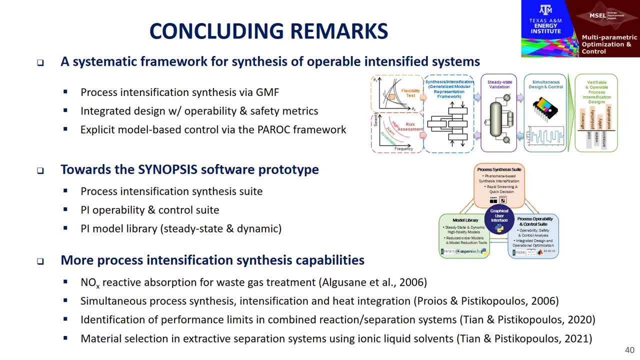 would like to talk about, But I gave you a synopsis of what is behind the synopsis framework And I will show you in a moment some glances of the software prototype. Obviously, there are many other in parallel intensification capabilities that go beyond what I described here, that can be found in other publications. 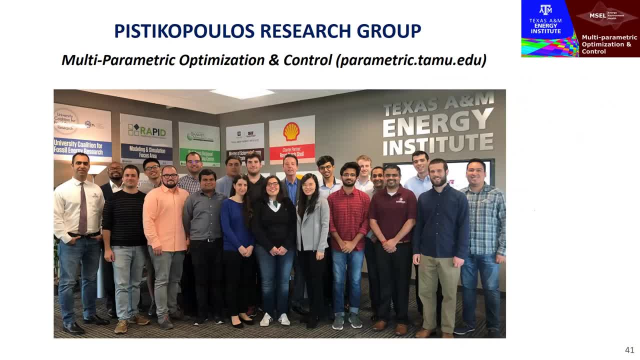 I would like to thank. here is the overall multi-parametric optimization control group. This is an old photo. we need to update it. Some people you know have graduated already and some newcomers have come, But that gives you at a glance. you know some of the key players in our research group here. 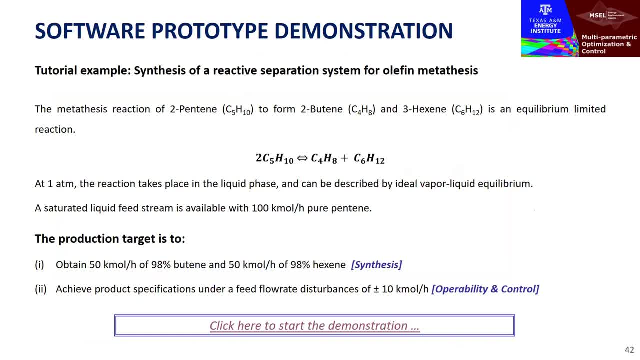 And let me close in the remaining few minutes to show you some of the aspects of the software prototype. Here is sort of a tutorial, It's. you know, the demonstration is pre-recorded, So you know, just to make sure that I don't press the wrong buttons. 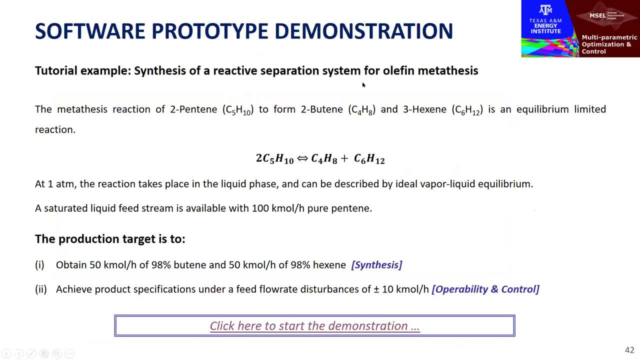 So it's a synthesis of a reactive separation system for allophen metastases. So this is the system. So you have a pentene that forms but-2-betene and 3-hexene, And the production target is to obtain what is shown here: 50 kilomoles per hour of 98% butene. 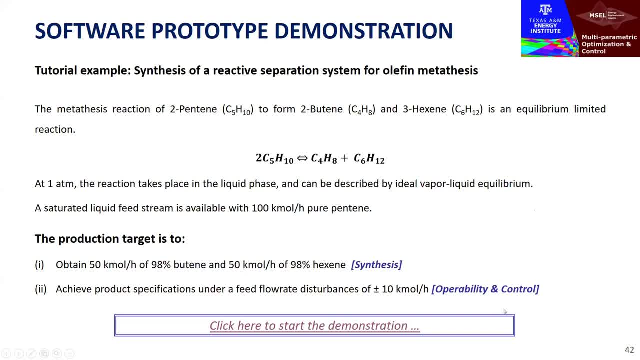 and 50 kilomoles per hour of 98% hexene And the synthesis level, And then you would like to achieve those product specifications. on the flow rate disturbances of FLAM-10 kilomoles per hour variability variations from this. 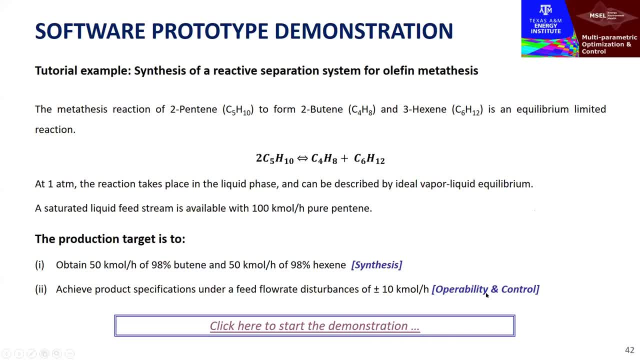 And we're going to demonstrate the operability and the control part of this. So the only I was promised that the only button I have to press is this one And everything else will come up magically. Ah, I need to press this button as well. 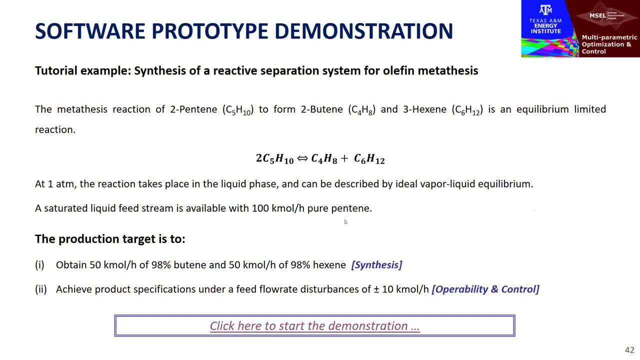 Okay, So here goes back to the. you know this is the front end. It shows the operability suite, you know, with the various functionality. Then if you press the button, you know it connects to rapid. I can stop it please. 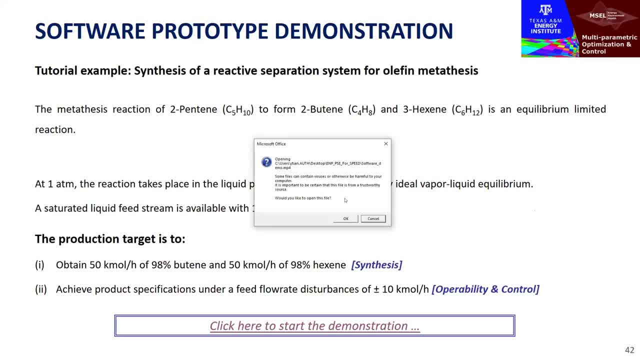 Yeah, So all right. All right, Let me restart. Yes, I was instructed that I can stop the simulation. Okay, Okay, So thank God, you can next to me. Sorry, Does it show? All right, We have a technical glitch. 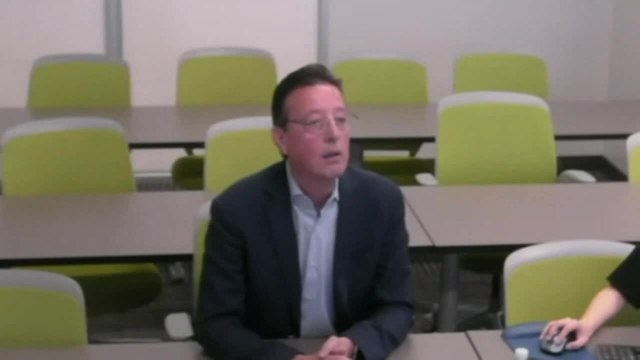 We're coming back live From Texas. Okay, So we're we're ready to go, So, uh, we're going to go to the next session, So we're going to go back to this one. This is the uh, this one. 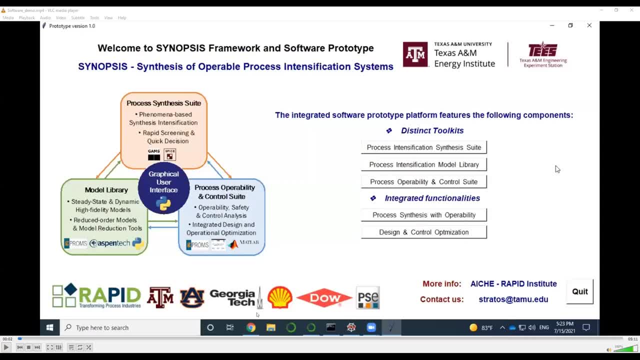 Okay, Okay, So we're going to go back to the next session. This is the next session. Okay, So we're going to go to the next session. This is the next session. Okay, so we're ready to go. So here you see the Oops. it goes too fast. Let me go back. 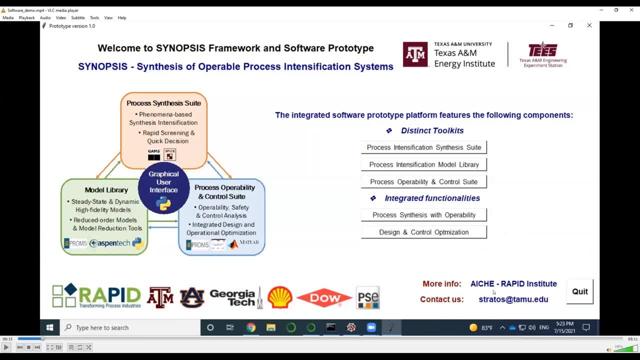 All right. so there is a functionality you can see here that you connect to Rapid Institute contact. so then you can see there is the front end here that connects you to the various toolkits. Then, for instance, if you go to the process identification synthesis suite, 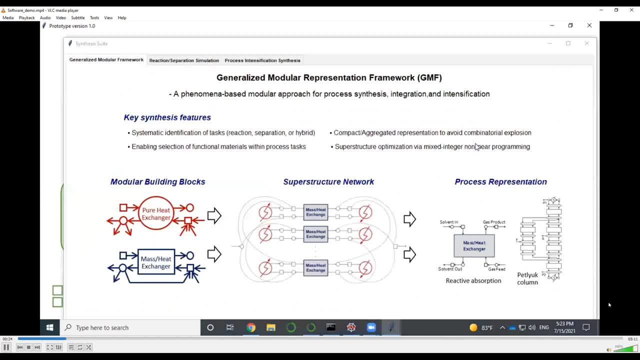 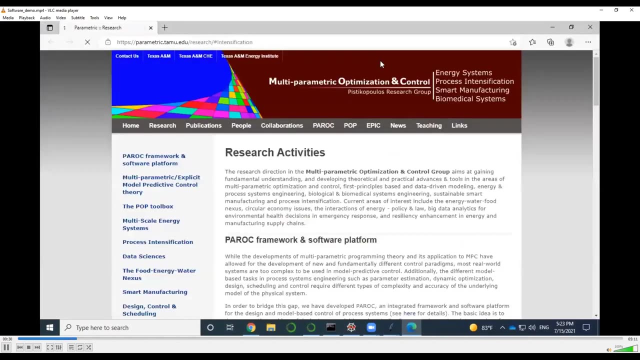 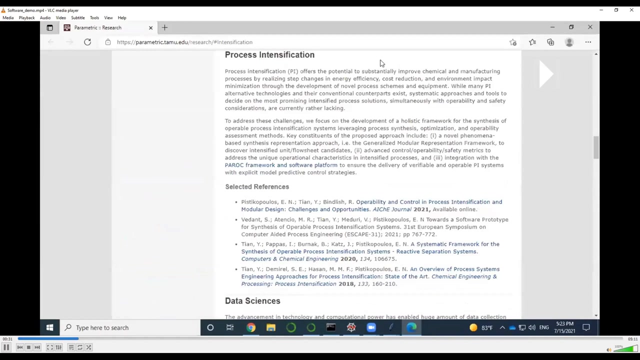 Did I press the button? Yes, Yes, Here it shows, you know, it gives a description, if you wish, of what this modular representation is. Then you can see the various components. It connects to our website for further information With key publications are listed. Then again you can see here the simulations. 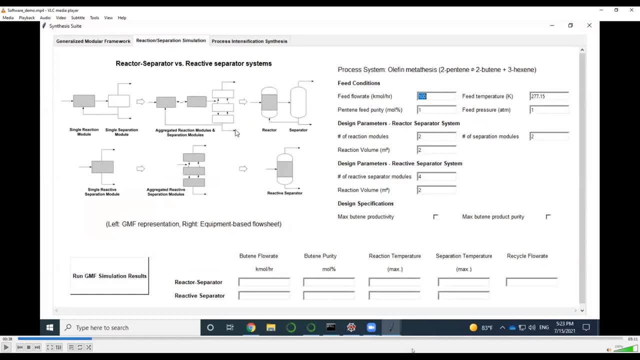 So it has two. So first of all it has like a background information with the button here. Then it goes into simulation because obviously you know, for people who are not interested in, you know, running the full scale optimization, they can play with different ways. 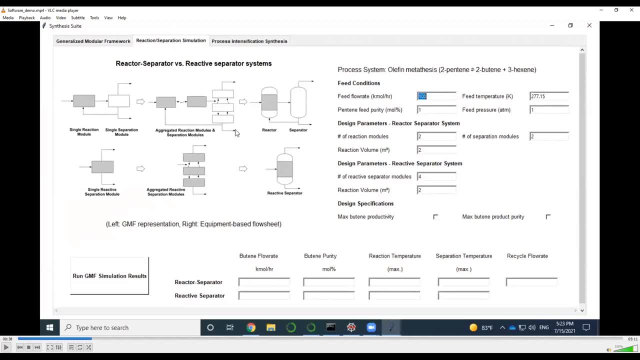 putting those building blocks together And start running the system signal in the simulation mode to see what they're going to get out. So here, for instance, you can see that they can generate all kinds of instances. They can change the fit conditions, the number of modules, and they can play with how many modules they can insert and see what comes of the system. 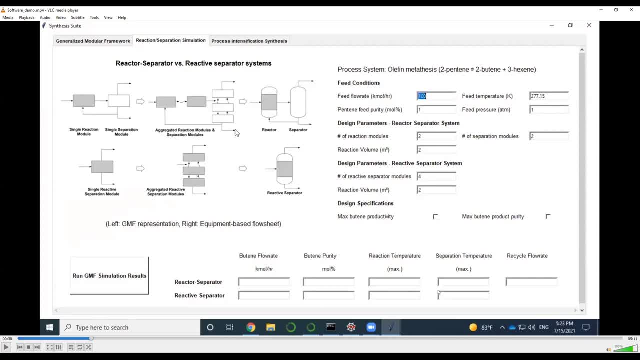 There is simulation. Everything will be populated as we navigate, Navigate the system. So, here you see, we insert various components, We put four modules, Then we have the capability to- I mean, we can- change those, And then we press the run button. 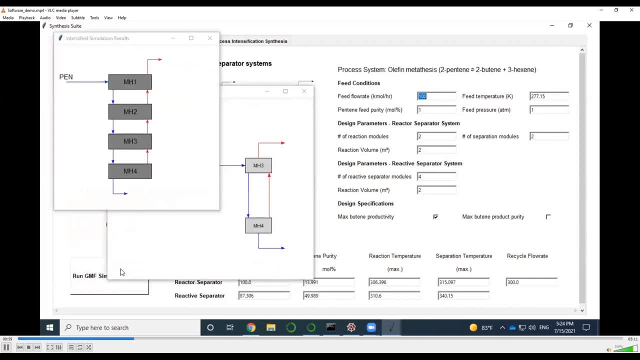 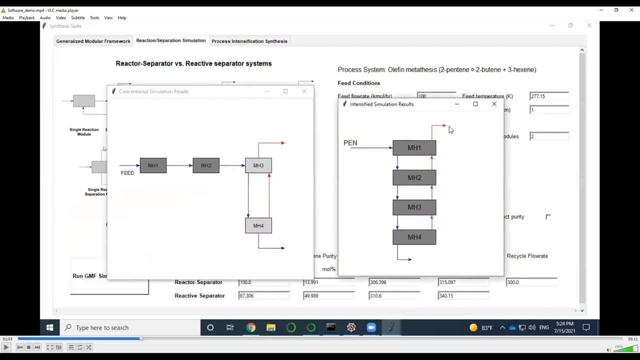 Hopefully it will be populated soon. Yes, And then you can see also on your screen, as shown here, that you know. so this would be the conventional simulation, Simulation of two reactors with a separation, And here you can see the reactive separation as well. 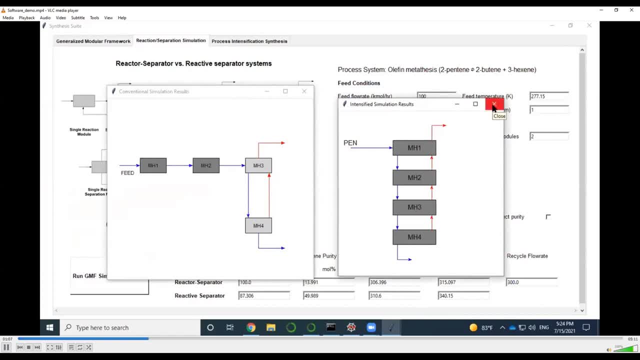 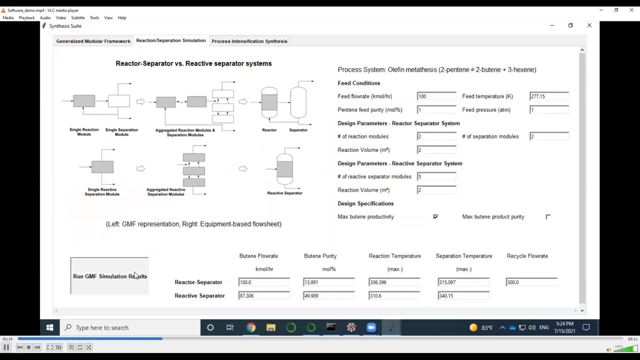 And then you can close this And you can go and perhaps change the number of modules. We're still in simulation mode. For instance, we put five modules And again you run the system. You can see the data here on your screen will be changing because of this. 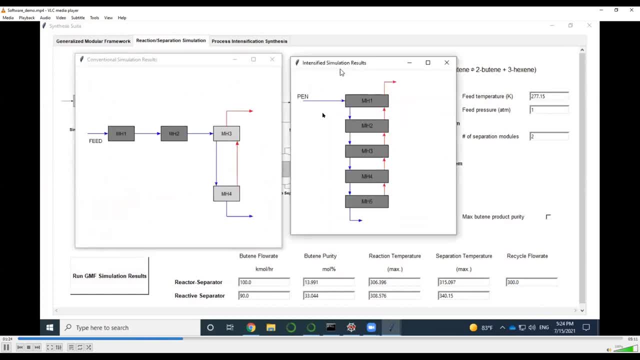 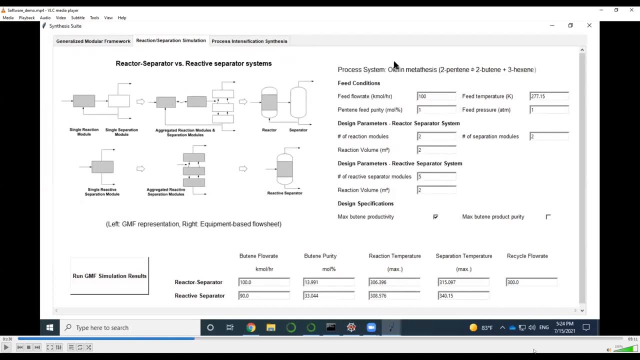 And again you can see the instances where you have the both the intensified system and the conventional system. And then you can go. And now, of course, the most interesting part is the synthesis bit, which I'm going to describe now. 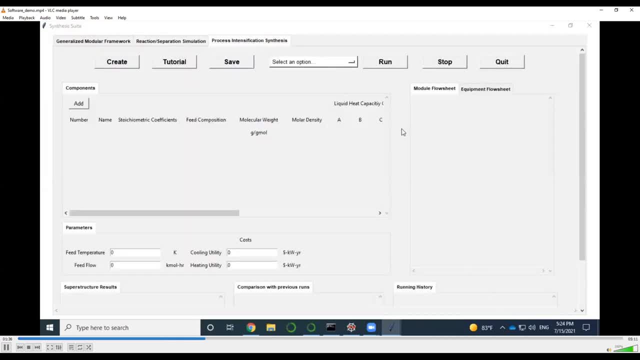 So after you complete. So here is where the synthesis mode now. So you have, you can add components, You can add parameters in a variety of ways. So, for instance, here we start adding the components. We have a library, It's normally. 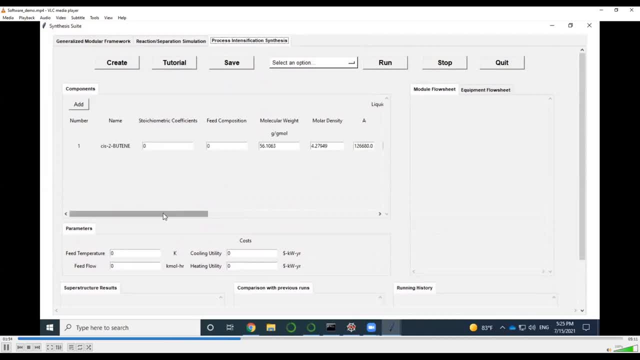 So you insert the three components here. The user has the flexibility to change parameters and so forth. You can see here some of those parameters And then you know we can have other parameters here as well, And then we can run, We can select. 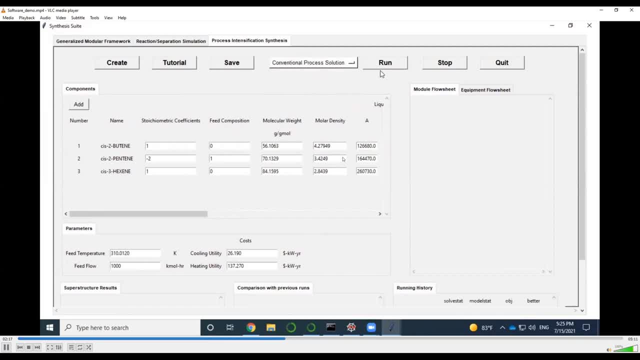 There are various options You can have, like a conventional system Or Intensify, So you can solve it in both: In a conventional way without any intensification, Or in an intensified way. So here you see the results of a conventional system. 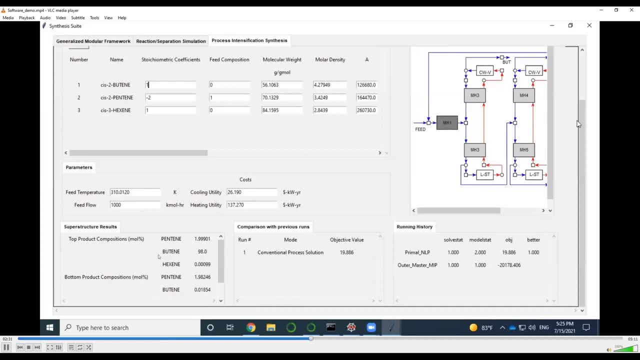 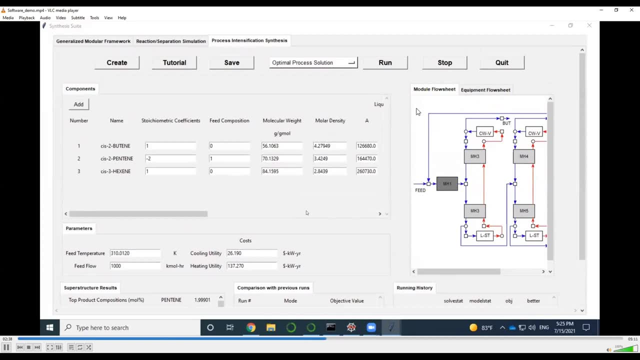 And you can see the bottom here, What comes out from the optimization, And then you can change this. You can go and do the, The, The intensified. Here is the result now of the intensified system. You can see now that it picks from the per postulated modules three: 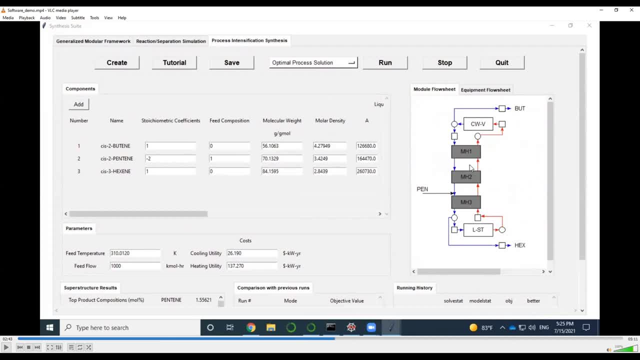 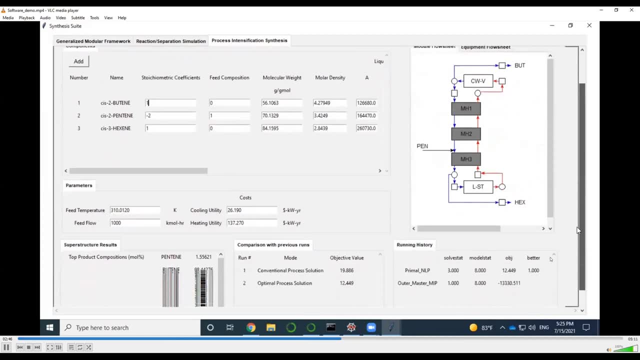 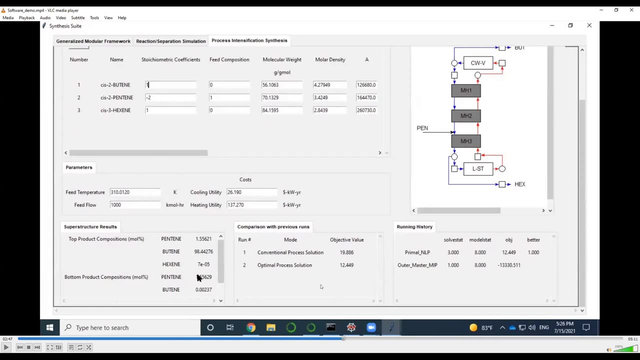 Plus the two auxiliary, only heat modules, And again You see here the results. You can see now at the bottom of the screen, If I stop here. You see on the left-hand side here is the outcome Of the optimization And you can have like the whole history of solutions we generate. 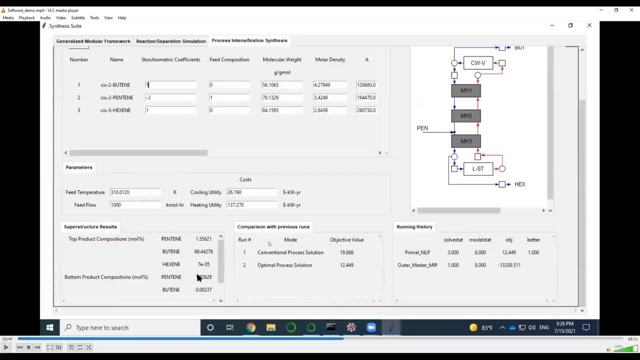 For instance- this is the conventional in terms of the objective- You'll see that the intensified system has decreased significantly The cost And in fact on the right-hand side here you can see the progress Of the Of the upper and lower bound in the mix integer optimization solution space. 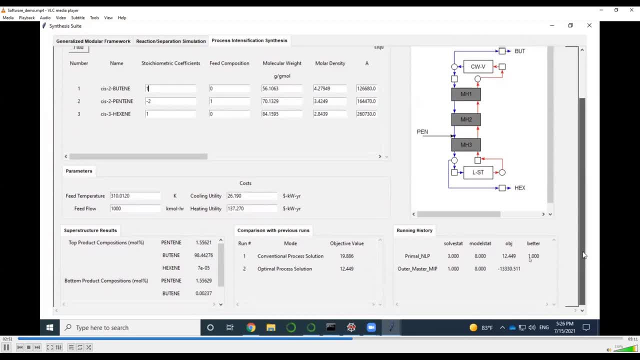 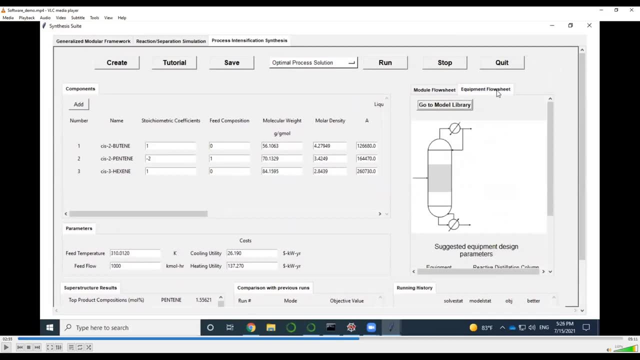 And Okay, So then You can transform all this. So this was the intensified Modular presentation. You can transform. now This is an equipment Flow sheet, And So here you see The The reactive separation. There are some. 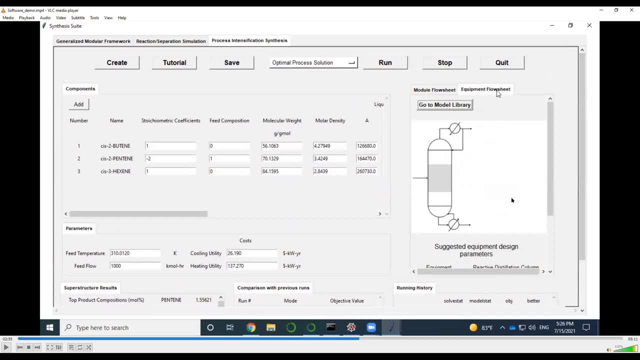 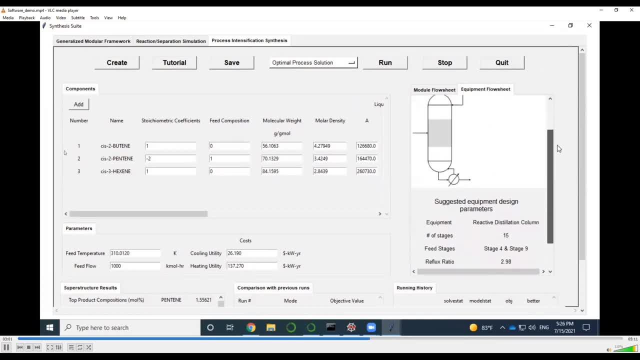 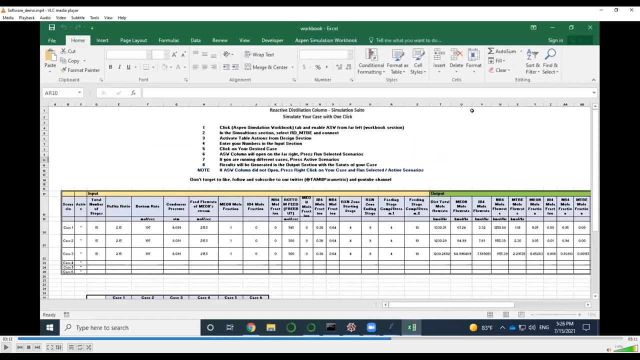 It starts. Okay, Yes, It's Now So you can see Their Suggested Design. hoch That Just to fit The equipment And flow And then Code To the model Library. The. 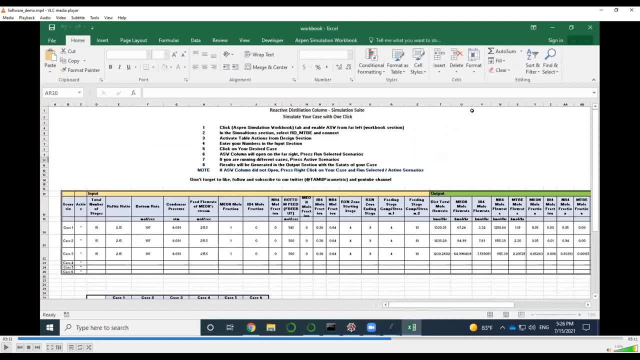 And Now screens A you know To translate option to insert parameters that, because you know not all simulate, you know that are inputs to the aspect, depending on what is the simulation medium. software that you, the user, is going to use here is for the aspect simulation, So we insert. 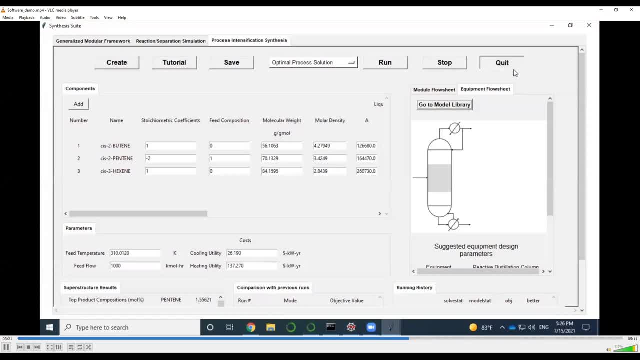 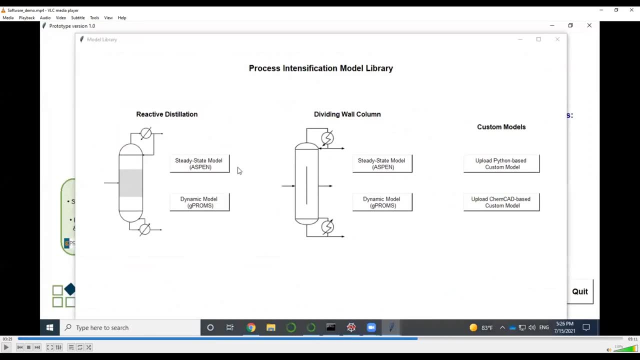 the information here and now. seemingly, the system performs the simulation and that is then stored as part of the model library. In the model library now, which is the second, we see we have validated models for certain class of problems and that can be customized and further extended. So we have 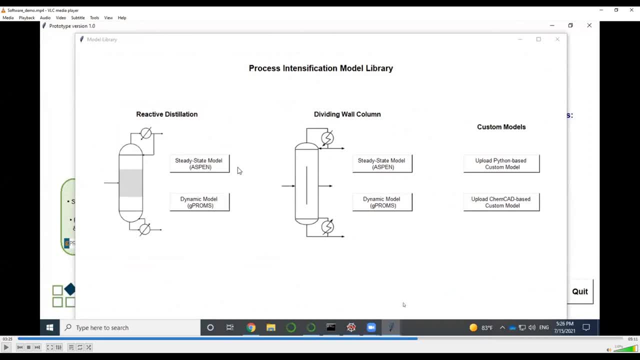 steady state and the current version has steady state and dynamic models in two software platforms of reactive distillation and divide. Well, obviously you know there's a whole battery, whole cohort of models out there that we can import from our other partners and so forth, But just 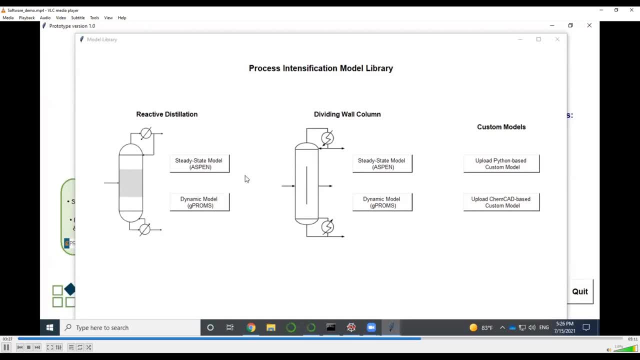 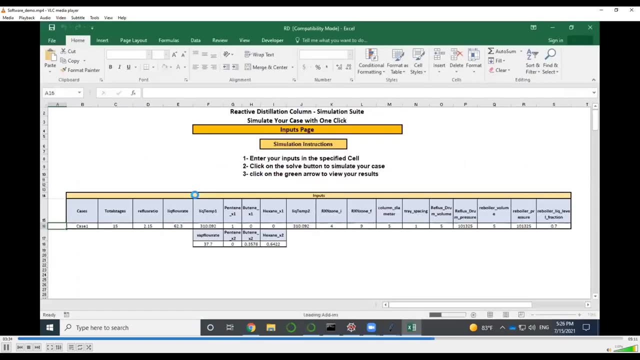 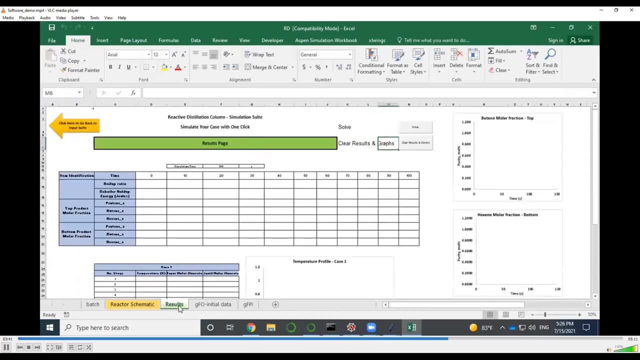 to support the activity. And then, for instance, now, the connectivity to the dynamic model. you know so, from the steady model you import, you extract the information and you now set up the dynamic model. And now we saw the dynamic. 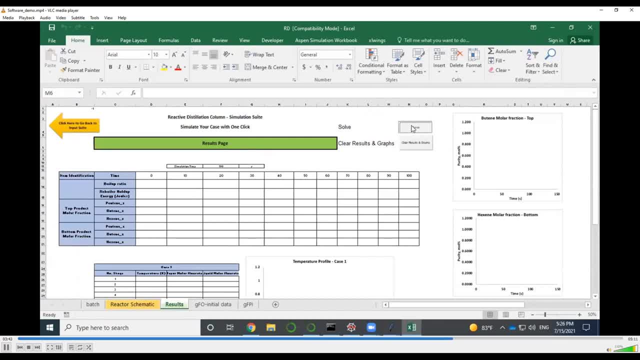 simulation of the reactive distillation. Now, this is a G from environment. you don't need to. the user doesn't see this automatically. It populates the various characters that you can see the graphs for this. So the temperature profile, the butene. 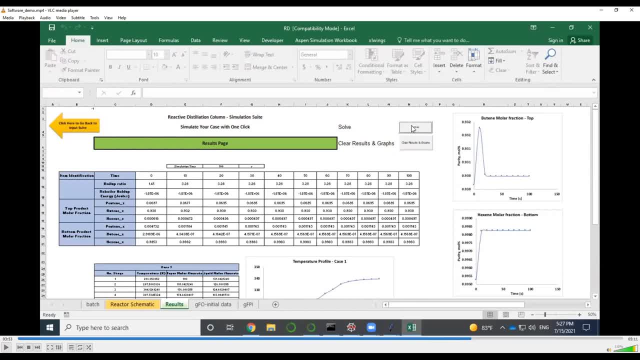 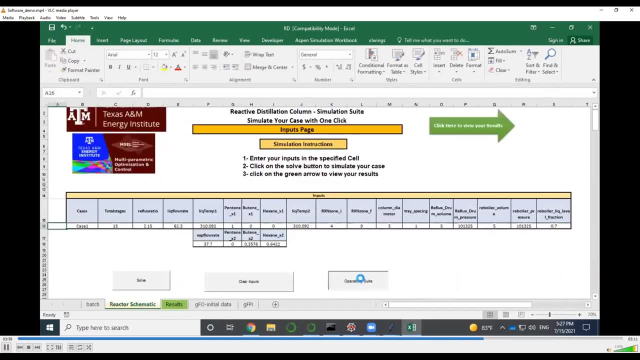 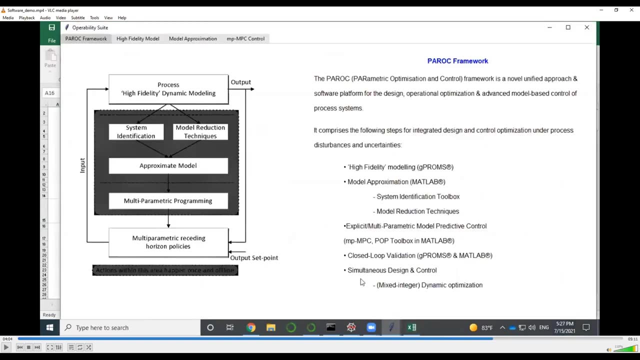 molar fracture and the exceeding molar fracture in the bottom. And now, with this information, I mean you can go to the operability suite. So now you're at the stage you want to check whether the system performs under very conditions. 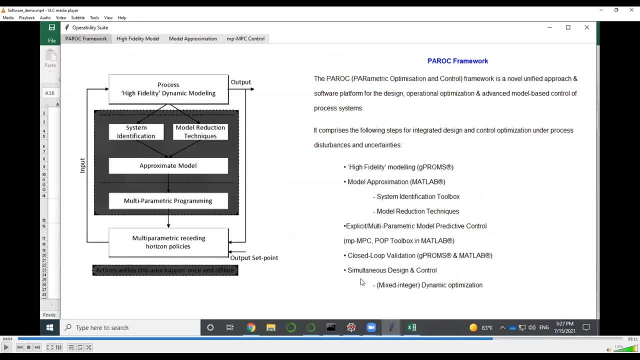 we can see there. So we start with the variability plus minus 10% A 10 moles. Now it goes to the part of framework. So we follow again. you have the. the part of the frame was across all these two very few days straight which gets a description of what the 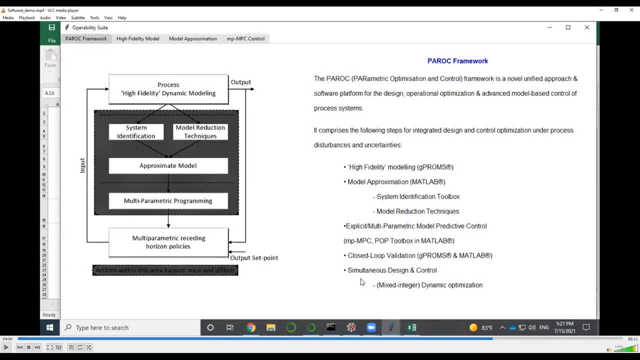 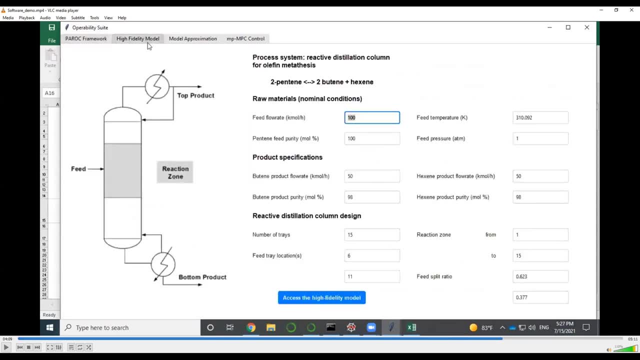 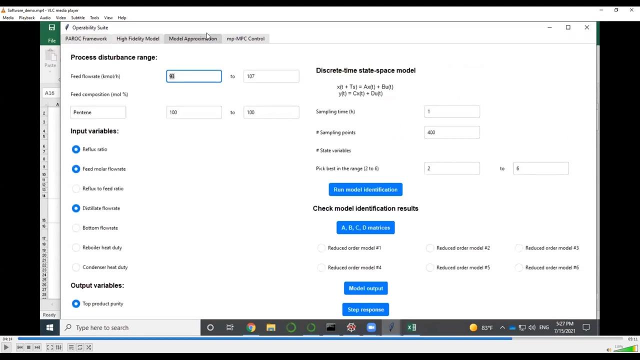 framework is all about, And so forth, with appropriate documentation. And then it extracts the high fidelity model from the ZEPROMs in this way, particular from the ZPROM suite of tools. It performs the model approximation here, Let me: yes, so, and it can perform various model approximations. So you can see here that there are 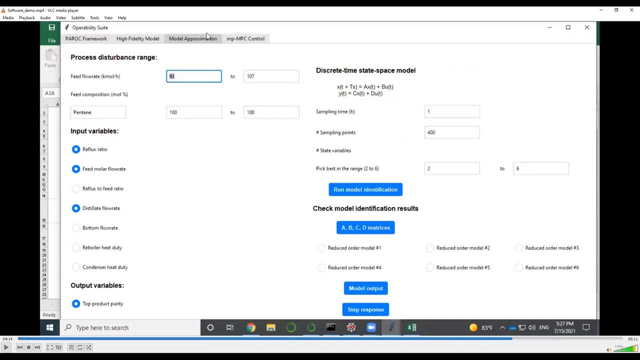 various reduced order models and then you can pick the one that has the better performance in terms of certain KPIs, how, in terms of the especially, you want to capture the product specifications as much as possible And then, based on this model, so you do the model identification step. 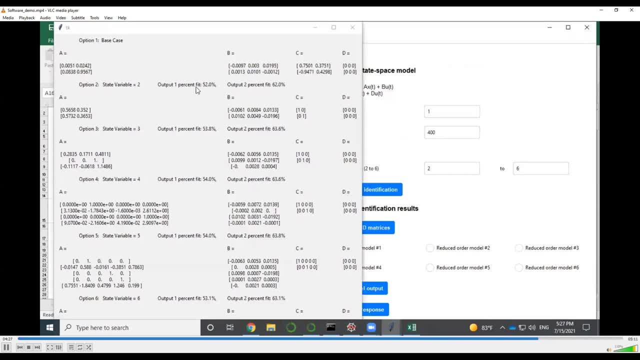 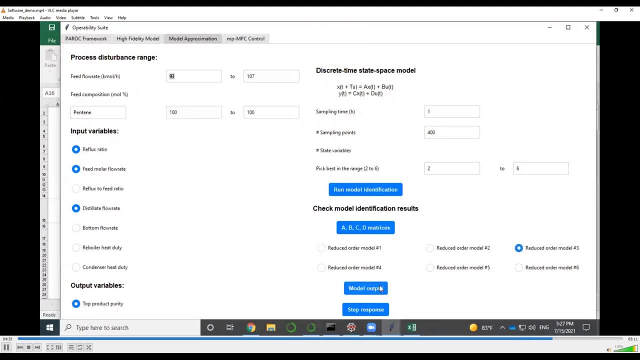 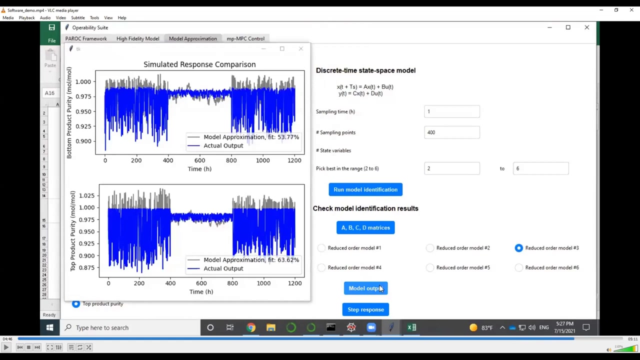 you recreate the matrices for the model, predictive control study- and based on this, then you pick the right reduced order model And then you run this. So now it's a closed loop simulation. So essentially it is. I did this yes, So no, here you see, actually, before you go into the simulation mode, 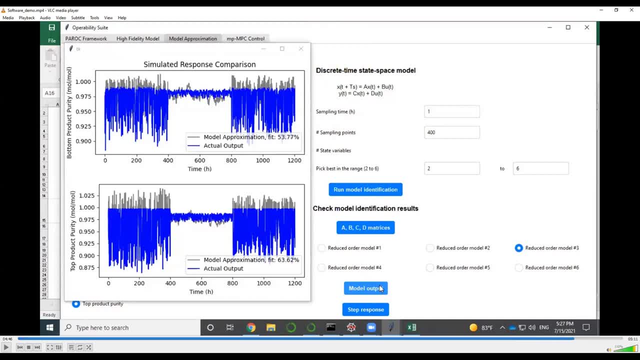 here is the comparison of the reduced order model compared to your original model. So you can see the level of approximation. So this is, you can pick the model that is more closely approximates your desired output And then you see the after you're happy with the level of the. 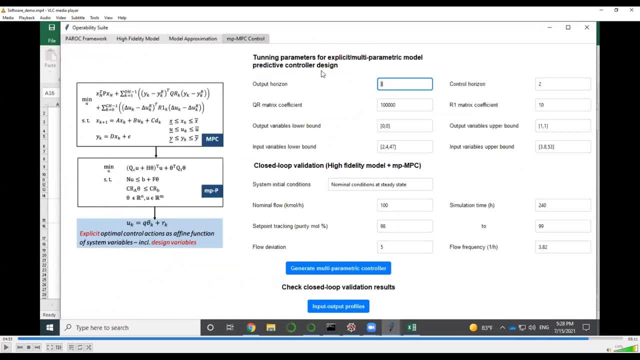 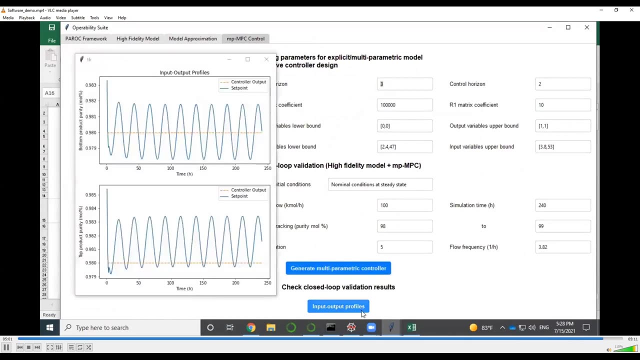 approximation. you derive the parametric controllers So, and then you incorporate those controllers in your original dynamic model and you run now closed loop kind of simulation with the parametric controllers And you generate here now the simulation. So now this is the outcome of the. essentially you monitor all the KPIs corresponding. 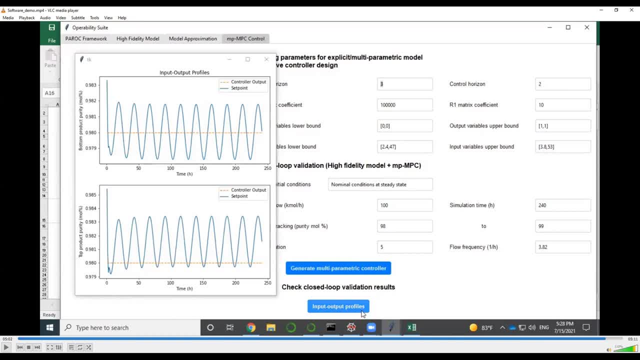 to the set point and the controller output. And because we have a periodicity here, you know obviously you are within the specifications and that is essentially a validated loop out of the full process. If you wish. when you started From posting the synthesis problem, then you validate it first through steady state, then you went into. 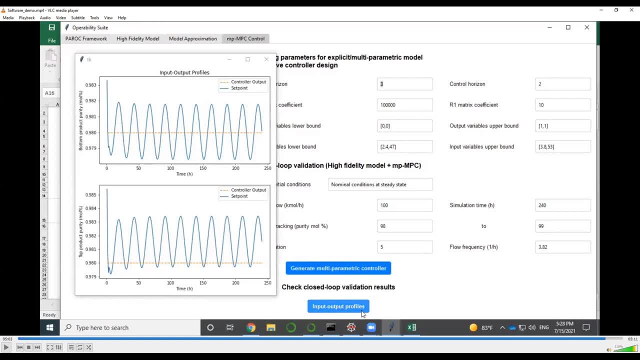 the model library, you converted the steady state into a dynamic model, then you went on to build the parametric controllers and then, with the parametric controllers design, you incorporated them into the or the original dynamic simulation, and this is the validation of that. this works. 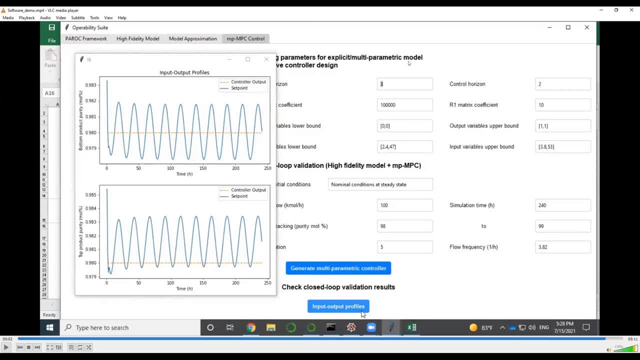 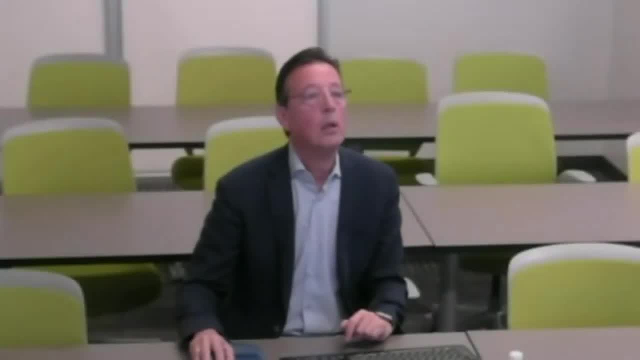 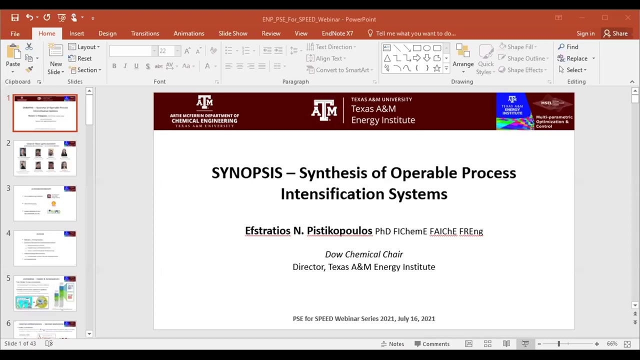 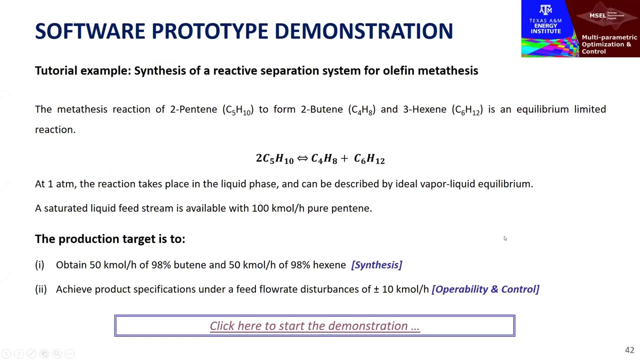 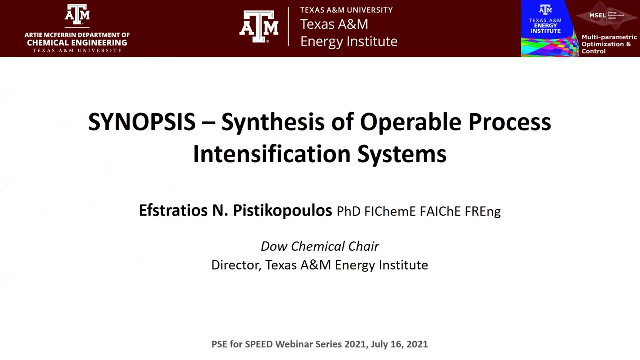 under the position. So if I close this, oh, and let me share my screen again, okay, and I think that essentially, Rafi concludes. you know a synopsis of the synopsis and you know at a glance demonstration of the synopsis prototype tool. So thank you all and I will be happy. 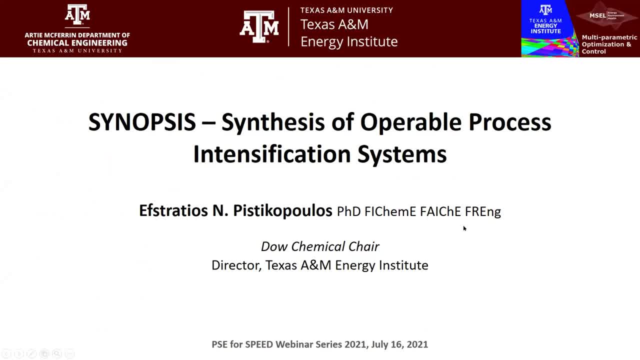 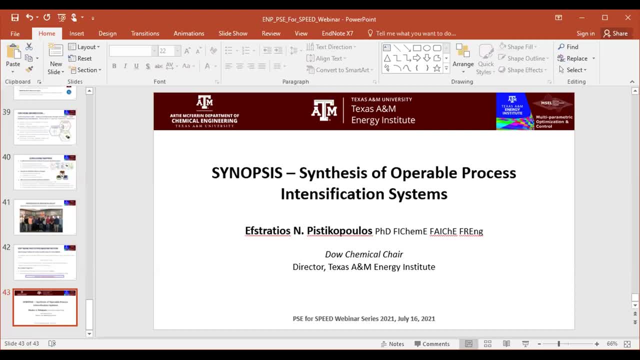 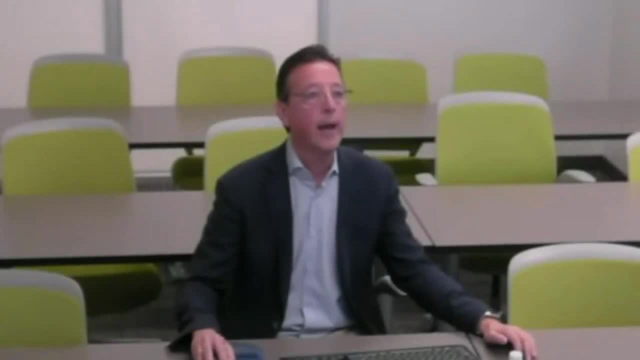 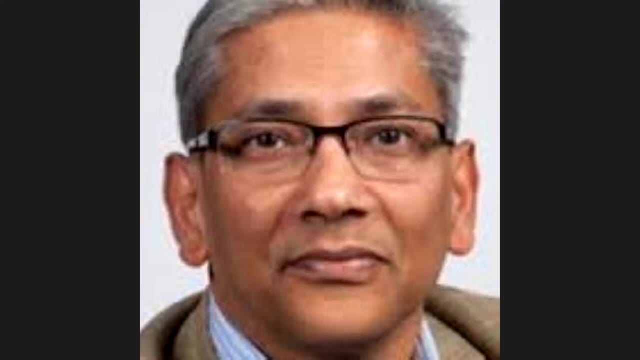 to answer any questions that you might have. Thank you, Stratos, for a very interesting lecture. Thank you so much. I stopped sharing. we can connect again if needed to for particular points. So if anybody has questions, you can either put your questions on chat or directly ask your question. 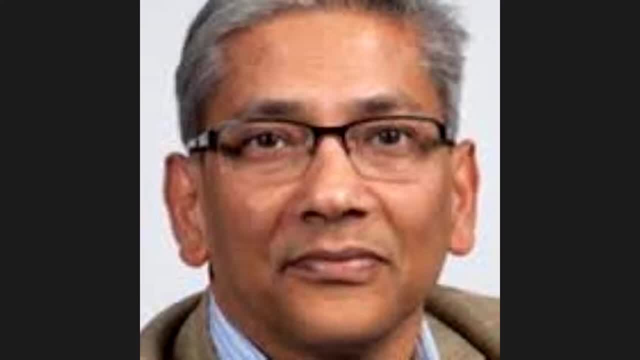 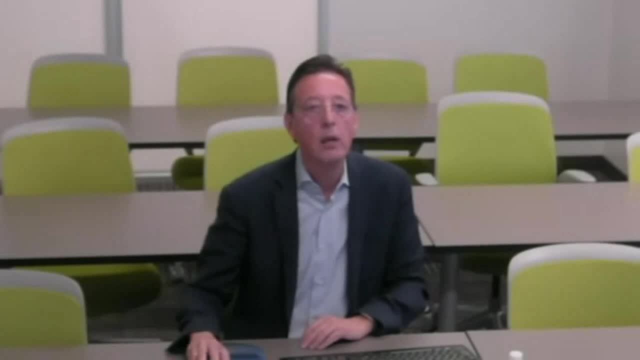 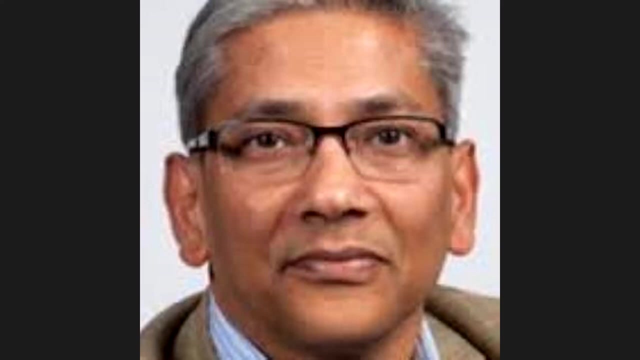 you would be unmuted if you show your hand. As I said, I will forward the slides to Jurafik and then you can distribute it as you see fit. Yes, thank you very much. Okay, so while others are thinking about a question, maybe I will ask one. 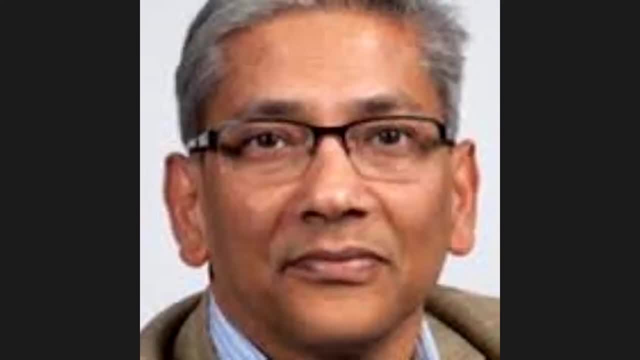 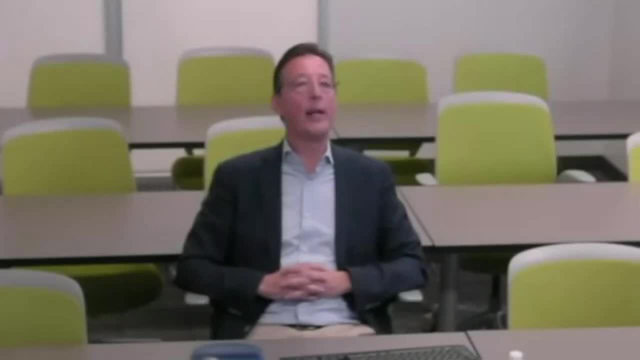 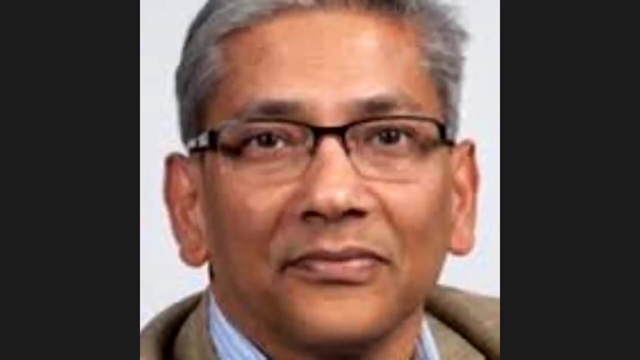 Yes, please go ahead. It looks very promising the tools you have put in. I think we are making good progress. let me put it that way: I think we are happy with the progress that has been made. yes, Okay, so when you want to solve a new problem, do you just give, let's say, the compounds that are involved and the reaction and everything else is developed, or what kind of extra information would be needed? 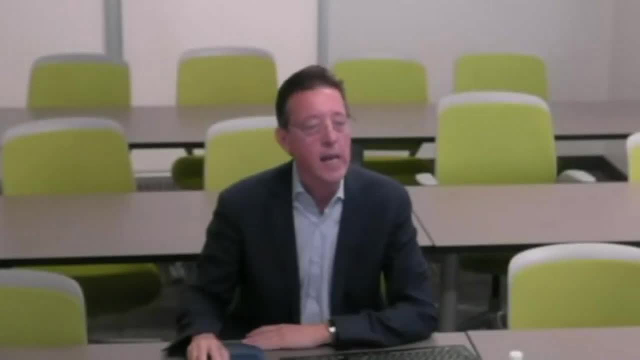 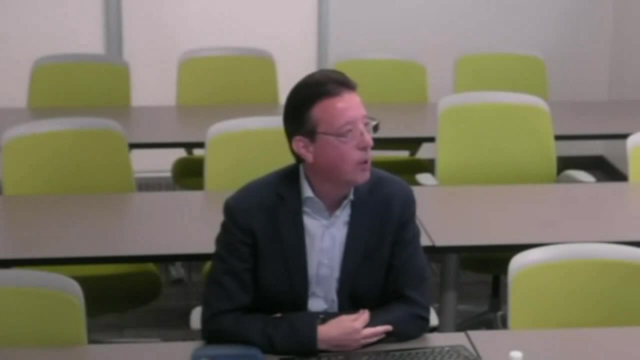 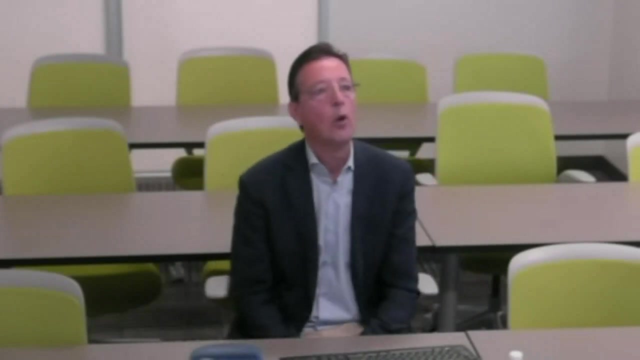 Yes, I think that's a very good question. That is a pretty So essentially the first release, the version 0.1, will have two classes of problems. One, the reaction separation type of systems. so essentially you will define the problem: vapor, liquid type of system. I should say 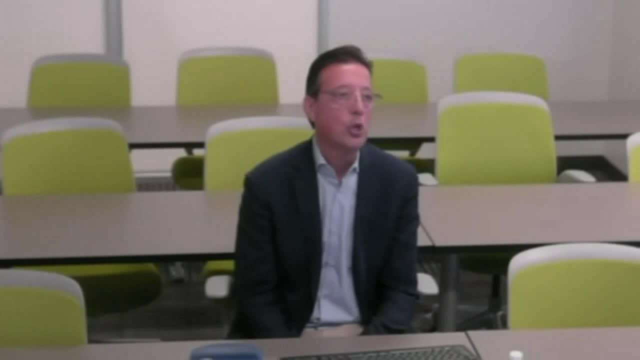 Right. It will cover conventional reaction systems, conventional distillation, plus any reactive distillation possibilities with input you know, like you know the compounds, or you can define the compounds you know. so, as we highlighted in the exam, 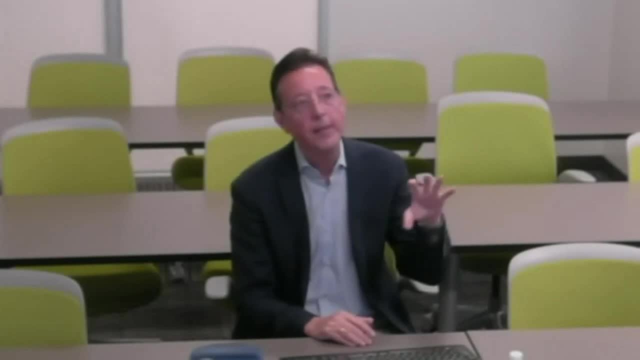 And it will also have the capabilities for all the three parts of the toolbox that I highlighted, such as we have the process synthesis toolbox, the model library, complete model library with validated steady state and reactive separation models and everything in between, and also the way to the operability suite. 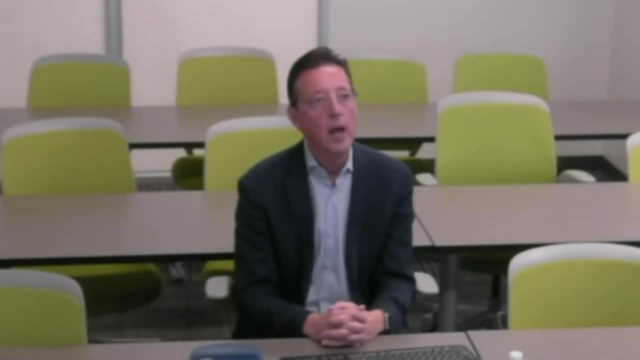 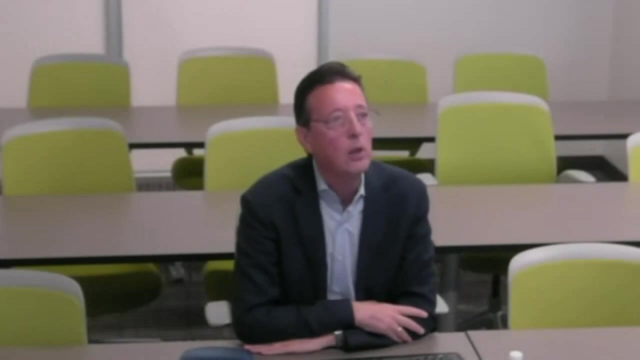 And it will also contain elements of the device. So that will be version 0.1 to show the visibility of this kind of framework and we will be expanding it as a function of time. you know it will depend also with the interest of rapid, you know. 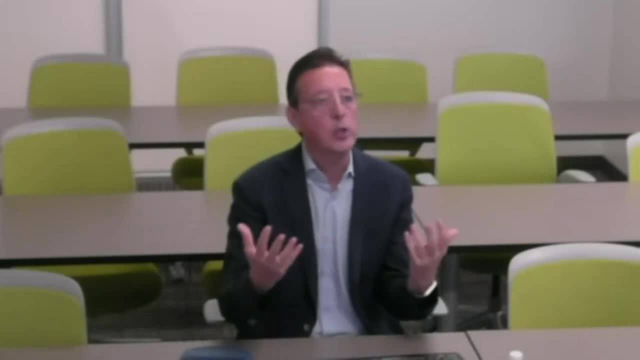 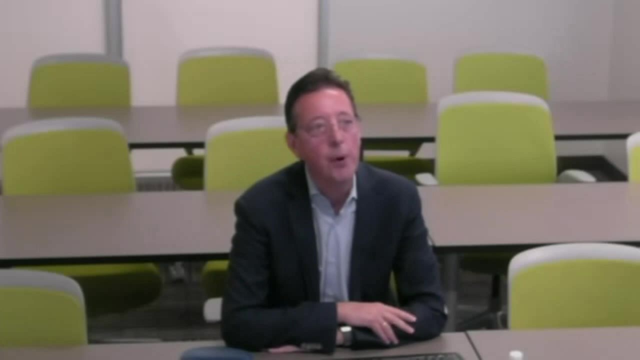 partners and also, you know, because, as you know, will depend on the, on the type of not only interest generated but all type of problems that people might want to pause from the processification problem so we can enhance the functionality towards that direction. 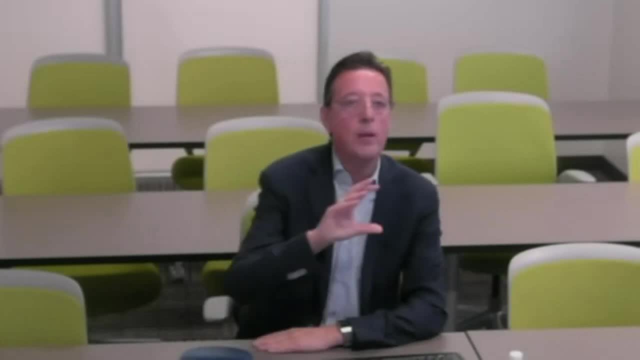 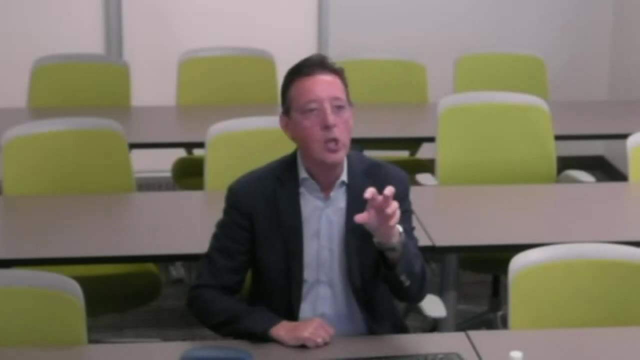 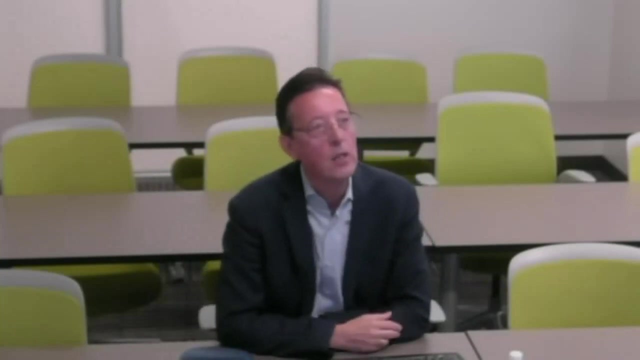 So now the emphasis is on the ensuring the automatic functionality between, let's say, from a synthesis to simulation. This is where the emphasis has been so far in terms of the functionality as far as the software flow of information. So this is where the emphasis has been so far in terms of the functionality as far as the software flow of information. 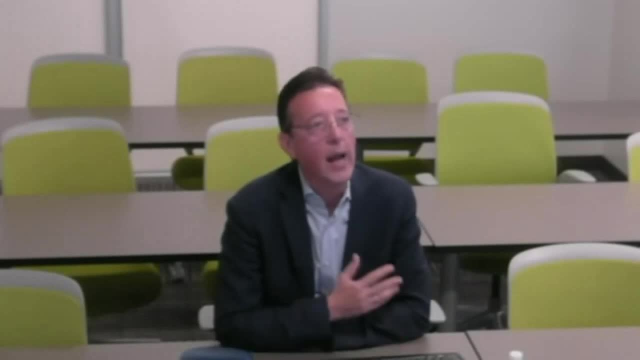 And then, clearly, we want to expand this thing- You know Agnostic, so it can be connected more than we're going to do growth spending. So, because it's these are the tools we are mostly, you know, using here, but obviously can be connected to other tools. So so this would. 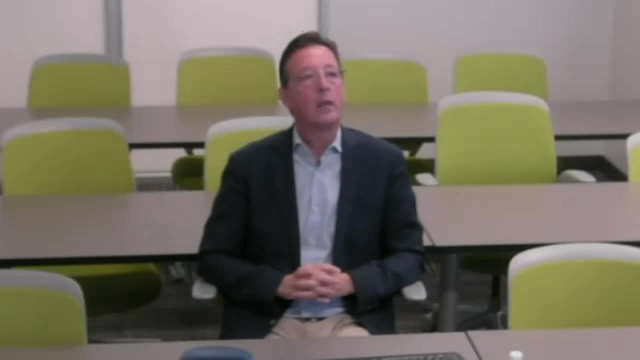 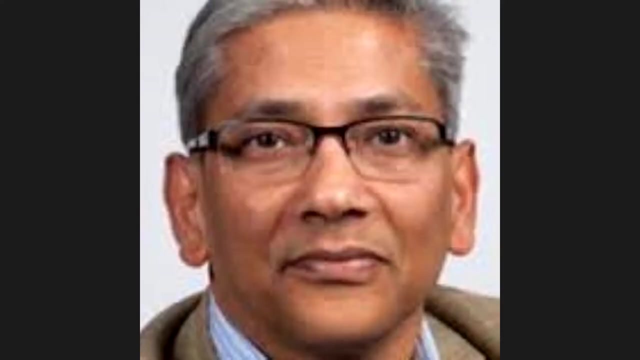 be like a Python based environment And ultimately, the synthesis framework should be only a Python based and the optimization through BiOMO, you know, will create the differences. So that's the direction we're taking, Very good. Are there any questions? Other questions? 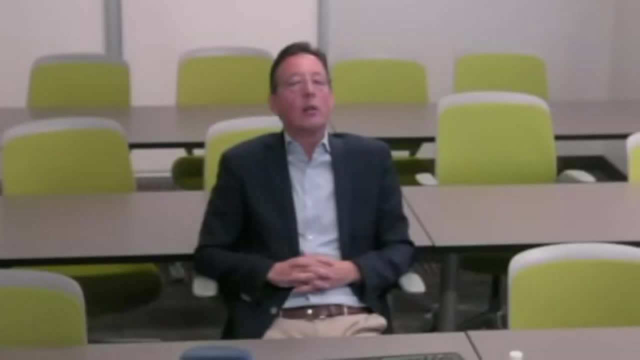 Must be very late in some parts of the world. Yes, in Asia it's probably very, very late, Yes. So I guess some people might be half asleep And I hope my lecture didn't make them full asleep. But you know, that's I can see in Malaysia or Indonesia, it's. 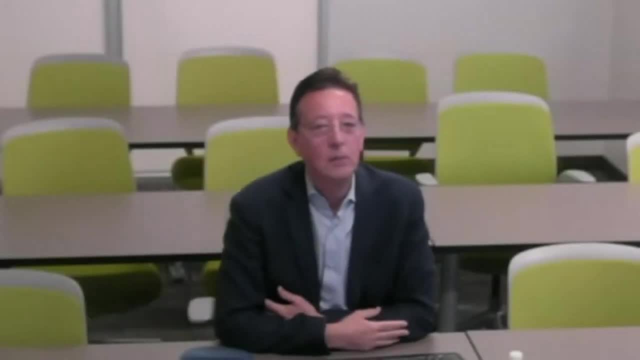 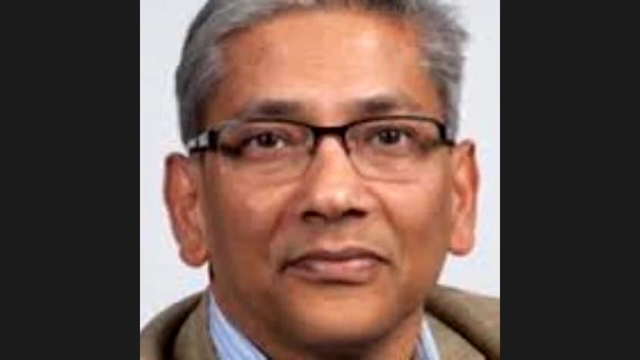 midnight. Thank you. Thank you for your interest. The lecture: Somebody has a question? Alright, bye, bye. Okay, so just one minute before you go. So this was the last of the of the webinars in webinar one. I do hope you got some idea of what is sustainable. 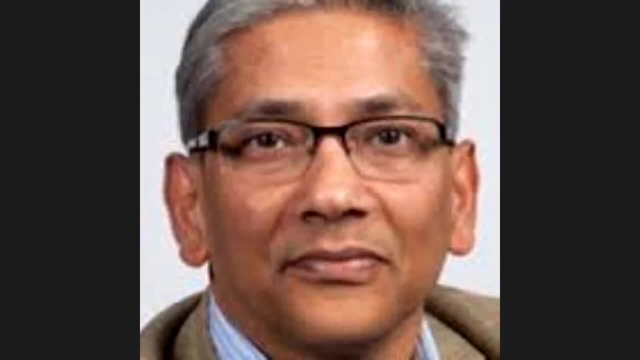 process development, And I think we could go on to the next one. Do you want to go? Yes, design. that includes, as Professor Pisticopoulos said, from synthesis to design, to innovation, to modeling, to control, to analysis, everything together And hopefully you have got some useful information and useful material that you can use if you. 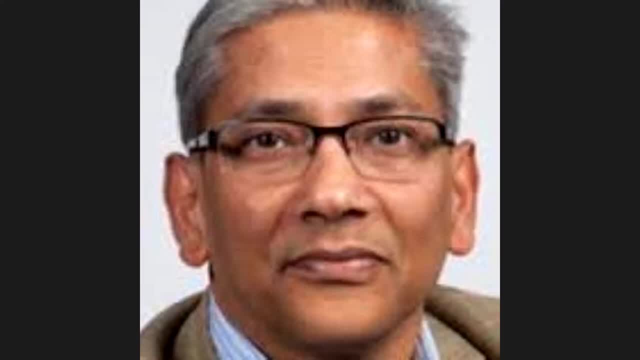 are studying. you can use if you are doing research. Hopefully it gives you some ideas. If you are from industry, hopefully you have found something that you can get from us all. the speakers, Professor Grossman, Professor Mario Eden, Professor Pisticopoulos and of